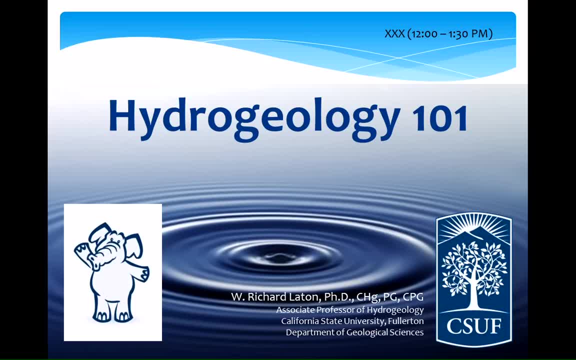 Oh nice, Get all the students up here in the front. That's good, Set an example. They're short, so I'll let them sit there, Especially Nancy here. you know she's like four foot one. Okay, we'll go ahead and get started here. 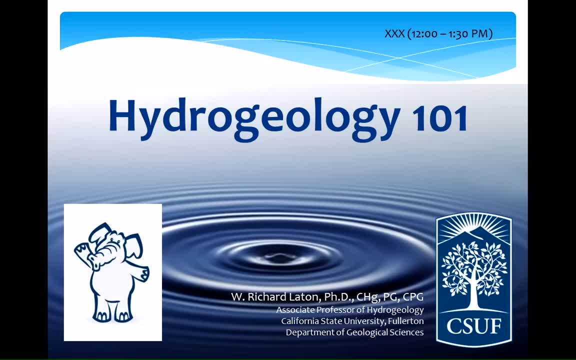 I'm Dr Richard Layton. I'm an Associate Professor of Hydrogeology at California State University, Fullerton. For those of you who are not from the California area, that's Cal State, Disneyland. We are about three to four miles away from Disneyland. 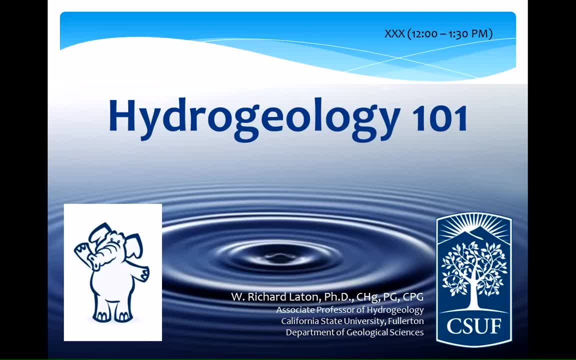 What makes Cal State Fullerton even more connected to Disneyland is they both opened in the same year And our campus is a really ugly campus. Apologize, sorry students, but it's a really ugly ass campus And it's big boxes. 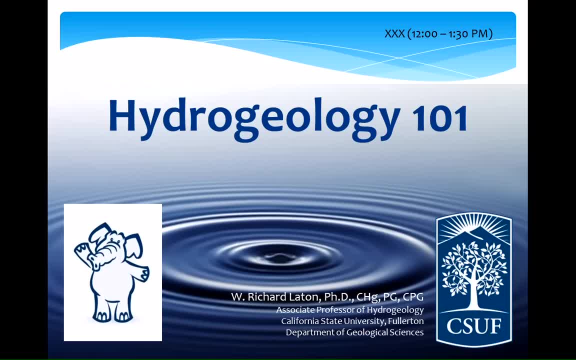 And so the rumor has it that when Disneyland came in, they unpacked it. We got the boxes, And since the state of California is broke, it makes a lot of sense, because I've never been wealthy. So, anyway, we're going to talk about Hydrogeology 101 today. 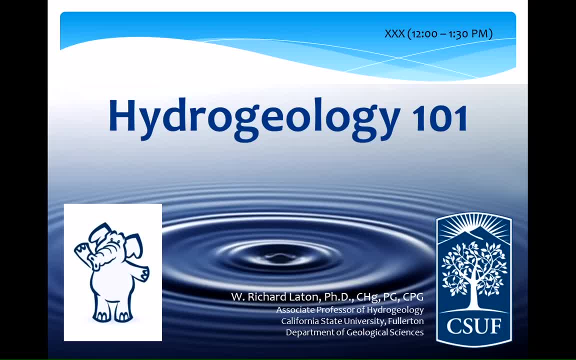 And I'm going to take you kind of through the water cycle. I'm even going to give you a little math, It's okay. And to give you a little history about me and how I got into this business. I have an oceanography degree from St Cloud State, Minnesota. 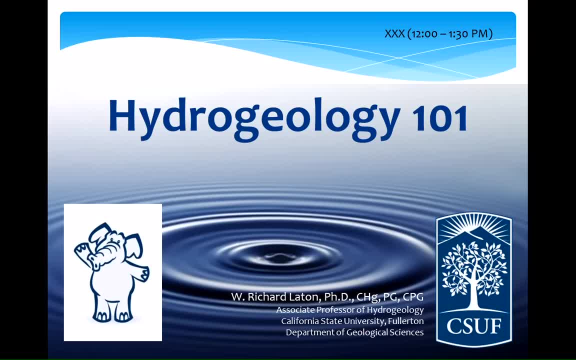 Now, if you know where Minnesota is at and St Cloud is in the middle of that state country, It's almost its own country. You cannot go to the state of California and say, oh, I'm going to go to the state of California. 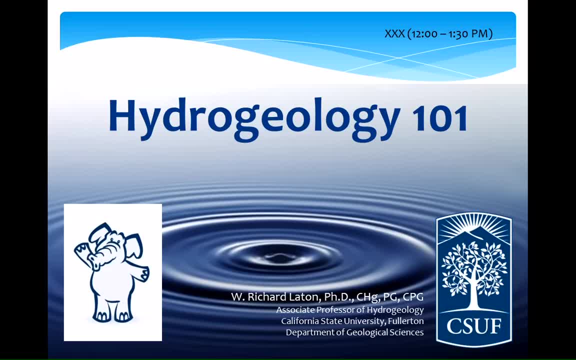 You cannot get further from an ocean than St Cloud, Minnesota. So when I went to apply for graduate school, nobody would take me And my GPA might have sucked, so that's okay. But somehow I found a group at Michigan, at Western Michigan University. 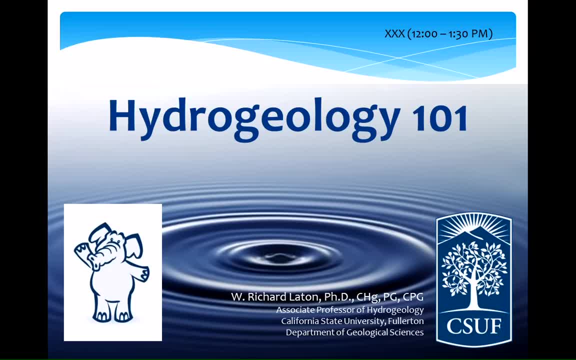 that took me in because I had some pretty good math skills. But what was more interesting- why you guys should pay attention here- is they had a drilling rig And they learned that I drove fork truck one summer for 3M, I was an intern at 3M and whatnot. 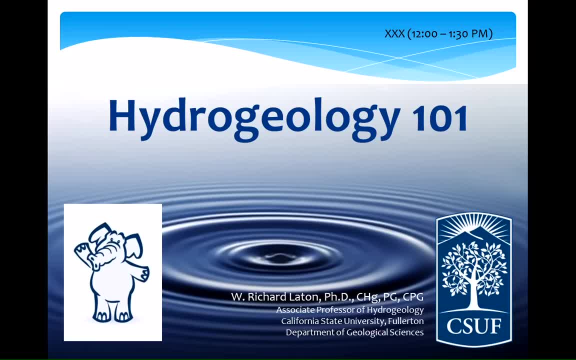 So I drove fork truck And so I went out with them one day when they were drilling some environmental monitoring wells for a thesis, And I lifted the sands of cement around and the sand and grout and everything And by the end of the day the head professor walks up to me and goes. 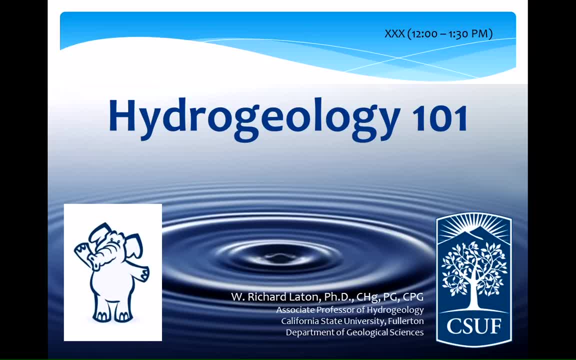 hey, I heard you drove fork truck. You're our driller for the next seven years. So in my graduate career I put in nearly 1,000 wells As deep as 200 to 300 feet, Most of them shallow. 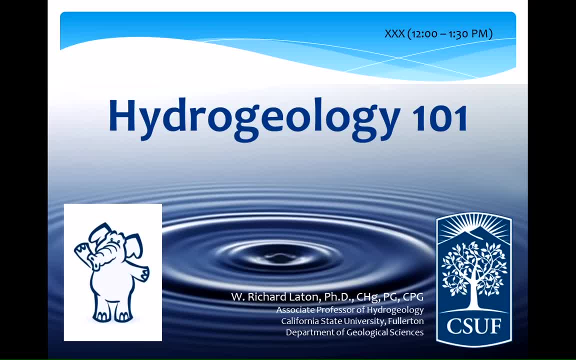 But I was their driller. Now how did I learn to do that? From a fork truck driving skill set I went out and talked to every contractor I could find and asked them teach me. So I actually got my hands dirty. 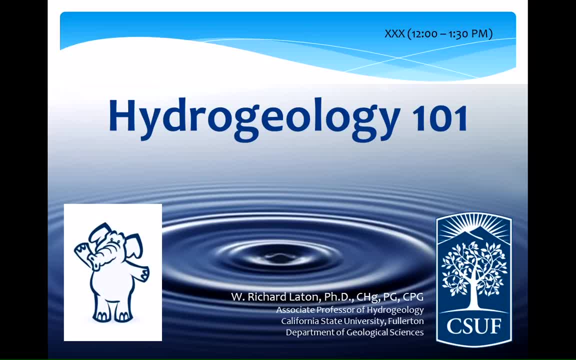 So when I got my doctorate I actually was in the drilling business, So I've actually done a lot of that. So I'm going to try to put into hydrogeology here the context for which it makes sense to everybody. So the objective today is just to get a better understanding of groundwater and groundwater principles. 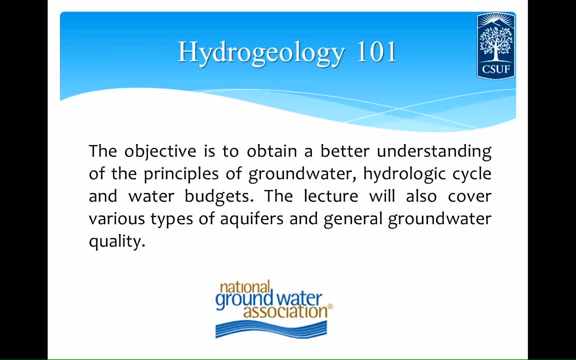 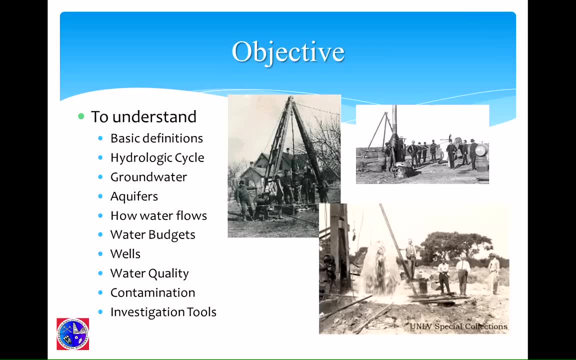 Like I said, we'll throw in a little bit of math. Nothing there, Nothing too serious, But I have to do that. I'm a professor And we're going to go through some different things associated with it, So hopefully today you're going to get some basic definitions so we all have the same verbiage to deal with. 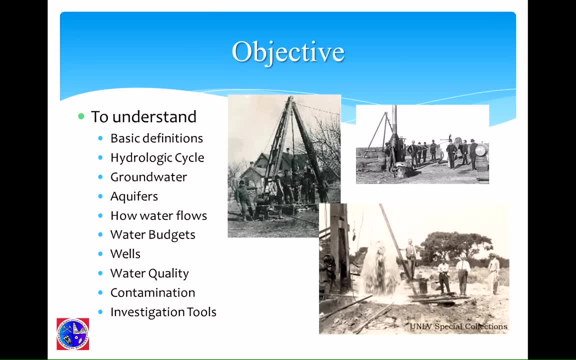 We're going to talk about the hydrologic cycle because groundwater is part of it, despite the fact our elementary schools don't teach that, Which really pisses me off. In the K-12,, groundwater is a forgotten subject, And yet it's what we usually get most of our drinking water from. 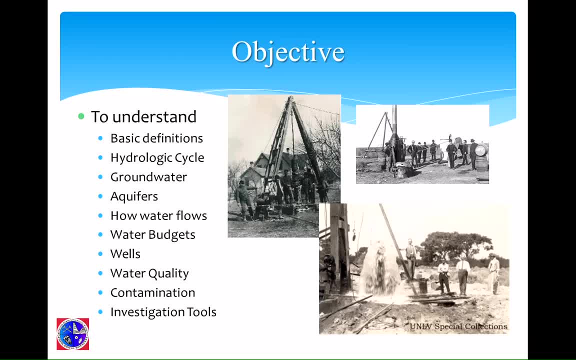 But we'll talk about aquifers. We'll clear up some mysteries about confined aquifers and semi-confined aquifers. We'll talk about some water budgets, some wells and contamination And then also show you some of the tools that we do to investigate things. 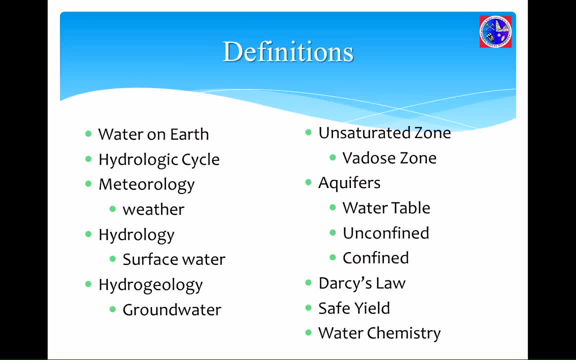 So some definitions, Just so we're all on the same page. We're the only planet with liquid water. Pretty important, The hydrologic cycle. What is it? We get evaporation, We get condensation, We get precipitation, And once it hits the ground it can either run off or it can infiltrate in. 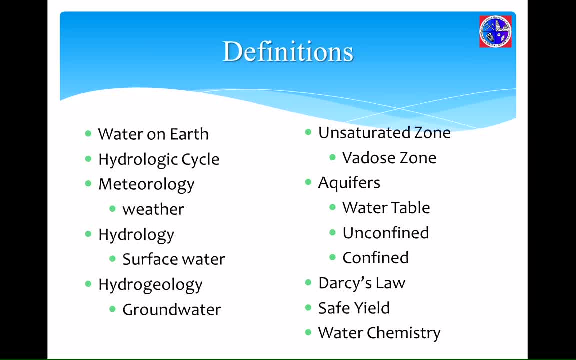 The stuff that infiltrates in is what's important to us, right, Because that's what groundwater ends up being. Now, where along that cycle happens, a lot of different things can take place Where precipitation happens and weather, And we're going to talk about some of the weather issues associated with it. 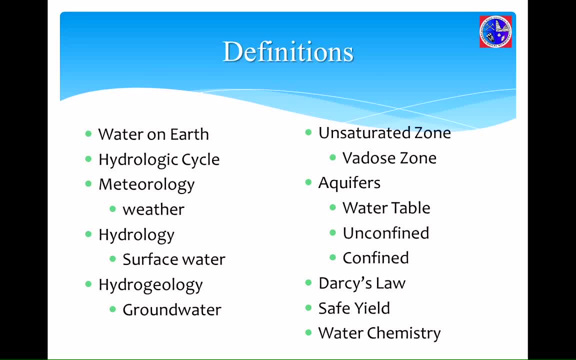 Hydrology. Why would we care about hydrology? And hydrology to me is the study of surface water. Hydrogeology is that water that resides in the dirt, But hydrology is connected To that dirt, for which the groundwater is connected. 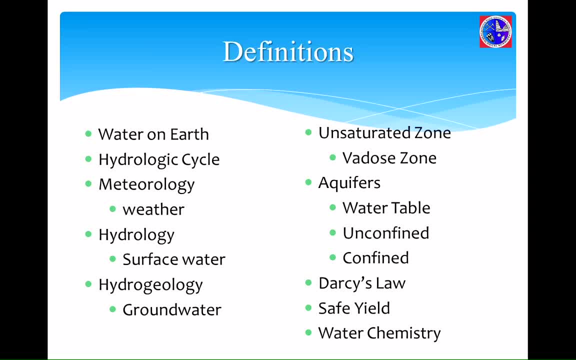 So there's a connection there And we got to talk about that Because that's certainly something that's a hot issue in a lot of states. How can I pump over here and not impact this? Okay, And I'm going to tell you some stories about how Orange County, California, deals with it. 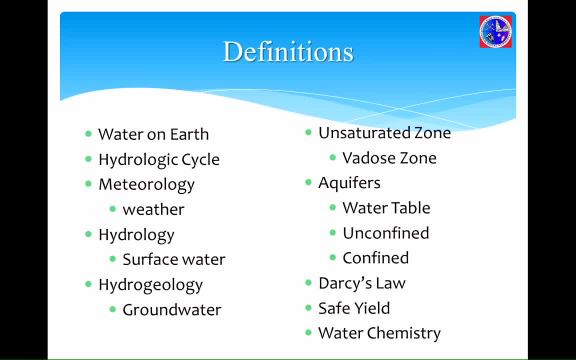 Unsaturated zone, That's that zone of air and water that resides above the aquifer. Okay, So there's some water in there, But primarily it's not 100% saturated, And we're going to talk about that. We're going to show you some slides and we'll talk about that a little bit further. 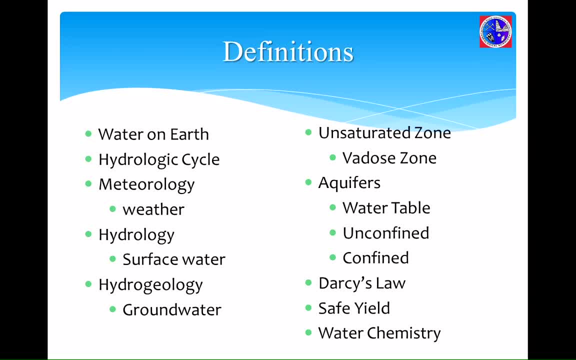 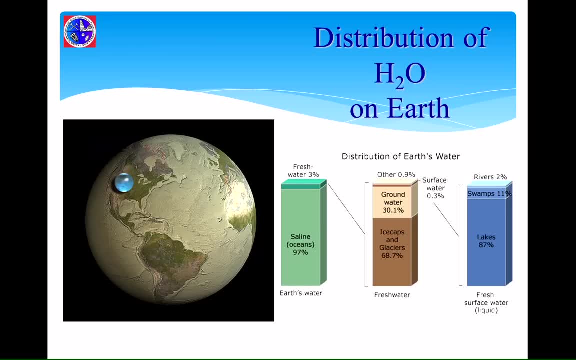 The water table. We'll define it. We'll define an unconfined aquifer and a confined aquifer. Then I'll have to throw Darcy's Law in there. Then we'll talk about a couple other things. So, distribution of water on Earth. 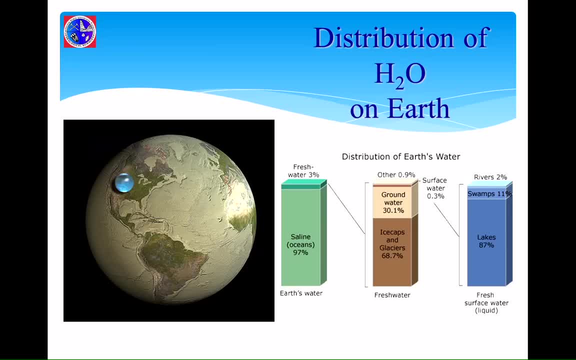 Most of the water, as everyone knows, resides in the oceans. Is it potable? No, So most of the water on Earth is not drinkable as is, So that narrows our little little piece of the pie that we're all interested in to pretty small. 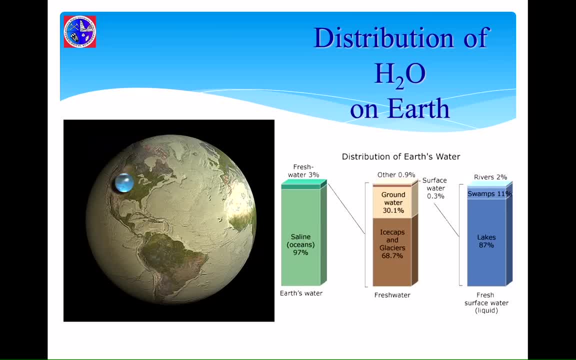 Okay, So fresh water is about 3% of the total water on Earth. Groundwater makes up a large portion of that, And I like this little slide here because right there is all the fresh water on Earth compared to the volume of Earth. 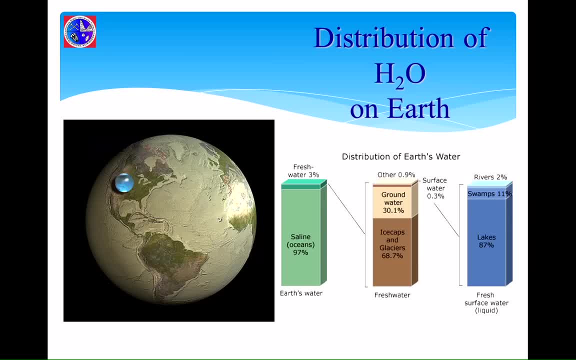 Groundwater. you can't see it, but there's a little tiny dot down here in one count. That's one county in Arkansas, okay, And that's really the potable water source we have for the whole world, okay. So it's pretty small. 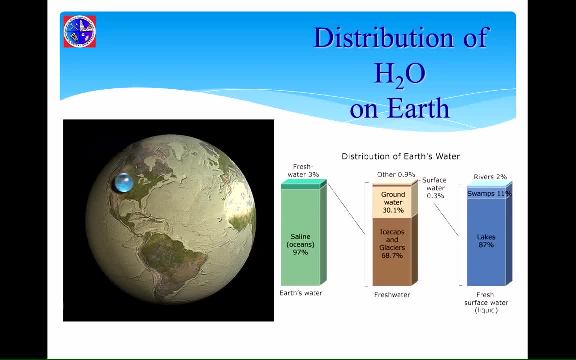 So it's something precious to us. Now it doesn't mean we can't take that salt water and desalinate it and do some other things to it, And people are doing that. They have to. Can't keep raising the population and keep your pie the same size and force everyone. 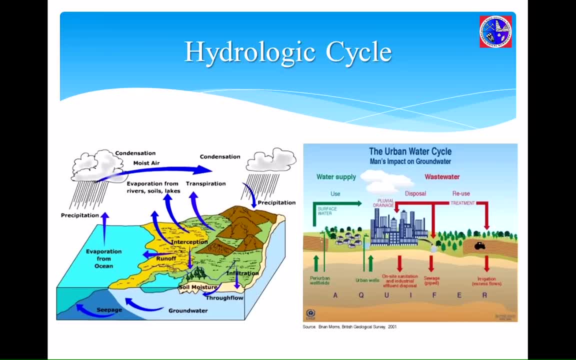 to live. So what is the hydrologic cycle? There again, we have open surface waters, We have water evaporates, We have plants that transpire and sweat, just like we do. Every time you sweat, you're taking liquid and you're turning it into a gas phase. smell: 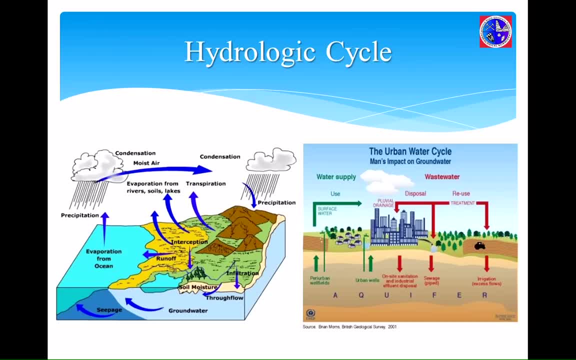 a little bit, But it's okay. That goes up in the atmosphere. okay. Water evaporates as pure H2O- okay. So when it evaporates, if there's any contaminants in it- be it salt or any kind of pollutant. 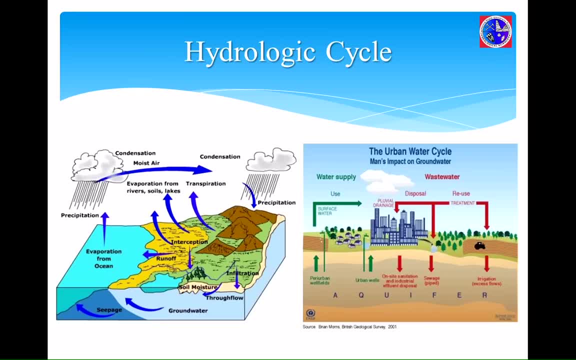 that's left behind. So when water evaporates, it only evaporates as pure H2O. That's why we distill water Okay. Once it gets to the air, it cools down and condenses, And at some point in time, oops, the weather system floats over, it condenses and it precipitates. 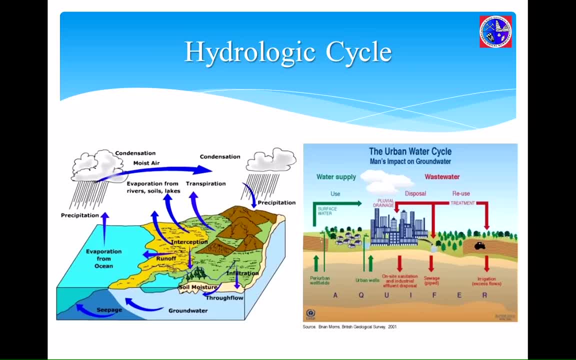 out And that precipitates out as snow, rain, sleet, whatever. It doesn't really matter to us At that point in time. we can have infiltration going into the ground and moving through as groundwater, or we can have runoff, And certainly runoff has some opportunities for groundwater recharge, but we're not going. 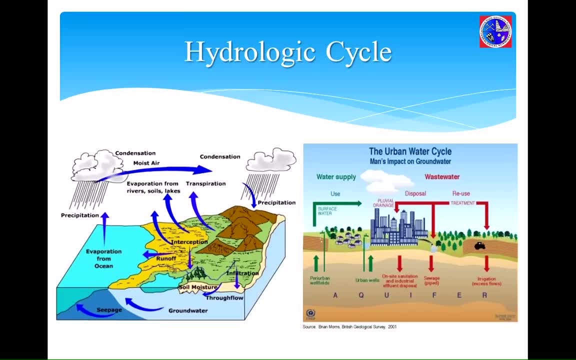 to talk about that. Okay, One of the things I want to bring up, though, which I think is going to be a bigger player as we move forward, is what I call the urban water cycle. Okay, The county that I live in has four million people. 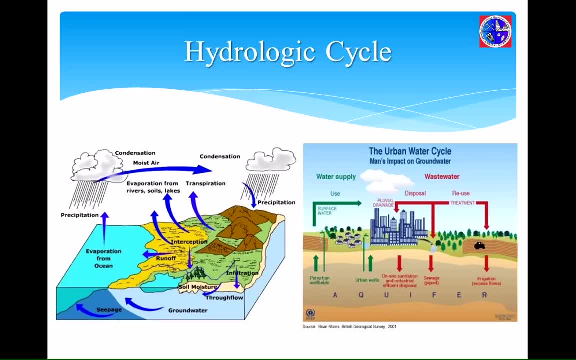 We recycle 100 million gallons of wastewater every single day back into our drinking water supply. Okay, A hundred million gallons of water that we treat and put back into our drinking water supply. Okay, A hundred million gallons of water that we treat and put back into our drinking water. 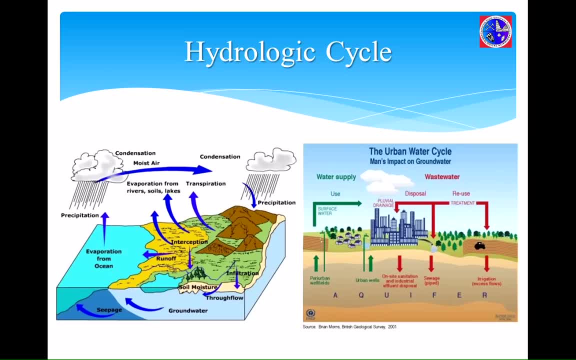 supply. Okay, A hundred million gallons of water that we treat and put back into our drinking water supply. All of the drinking water we have in our county is groundwater. We pull it out with pumps and wells, but it's all recycled water. 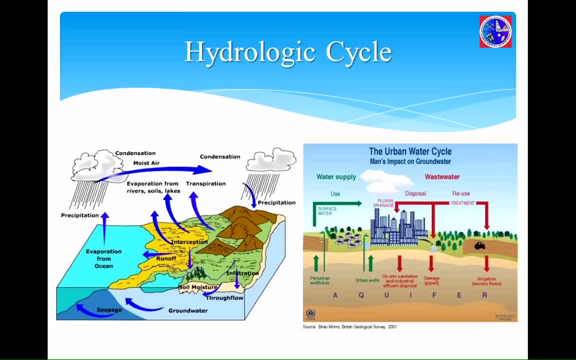 We're 100% sustainable in a desert. What's going to happen is we're going to start seeing people start using their water for whatever purpose, having that go back in the ground, and then we're going to pull it back out as some kind of usable. 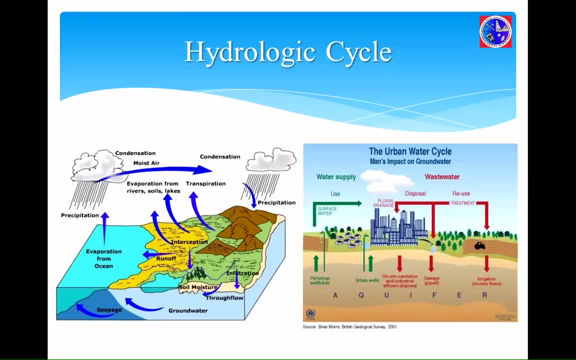 Now we have to treat it. That's going to happen more and more. One of the issues that came up was somebody was talking about Minnesota. Anybody here from Minnesota You're welcome. Good, we can make fun of them, right. 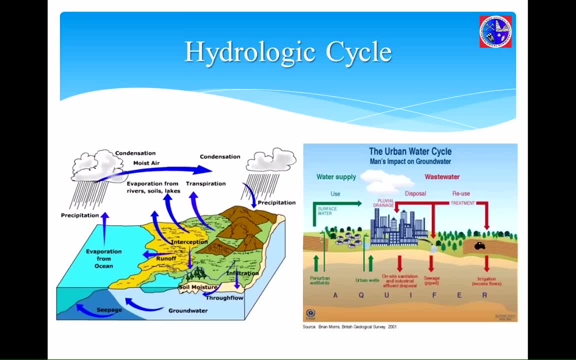 It's Minnesota. you've got to make fun of them. Land of 10,000 lakes. What's their problem? They're running out of groundwater. The land of 10,000 lakes. how can you run out of groundwater? Every one of those lakes is tied to the groundwater system. 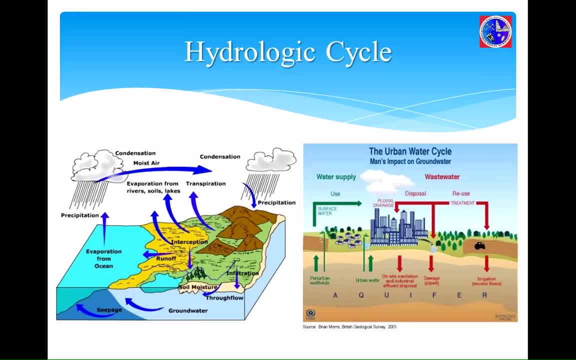 How can you be running out of groundwater? What's their water cycle? They pump it up, they use it, they put it in the Mississippi River and give it to Iowa- Anybody from Iowa? I can make a lot of fun of the Midwest. 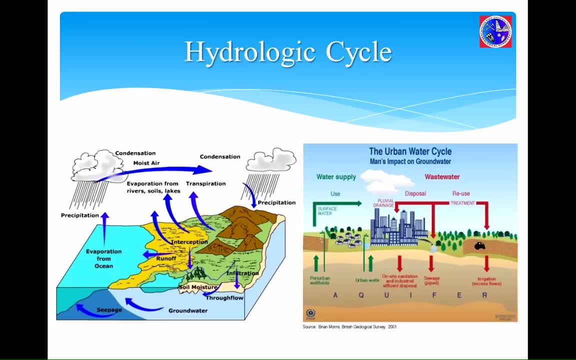 This works out well, So they just give their water to Iowa. Well, they already paid to pump it, They already used it, paid to treat it and then give it to Iowa. Why in the hell would you do that? Just put it back in the ground in Minnesota and keep it. 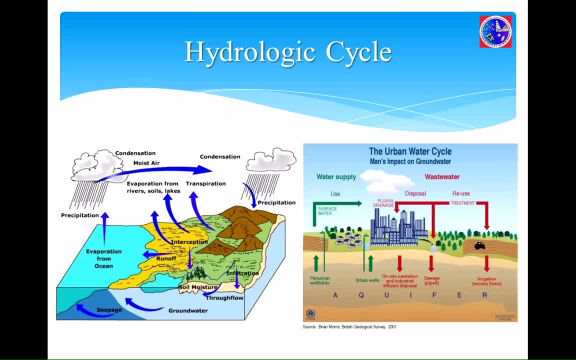 And that's something they're going to have to look at. So we're going to take, rather than letting that water all go down the rivers to the ocean, we're going to actually start short-circuiting that system because it's something we're going to have to do. 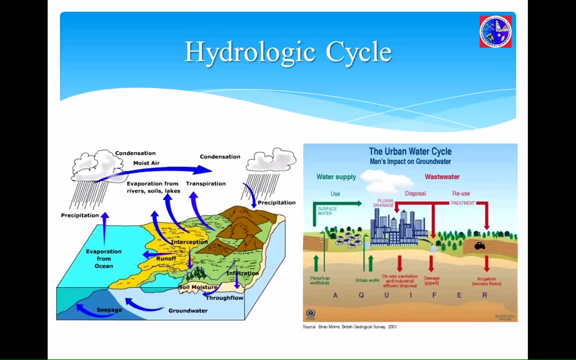 It's more sustainable. We're already paying to treat that wastewater. Why not reuse it again? And you can do this on a private property with a single well as well as everything else, because of what we've been doing right. You have your septic tank. it goes to Leachfield. 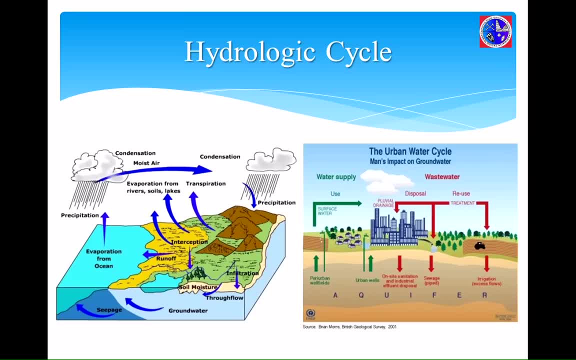 Where do you think that water is going? Right back to your well. You pull it back out. Now. it's been filtered and cleaned by the time it gets back there, but it's the same water. It's like my eight-year-old daughter. 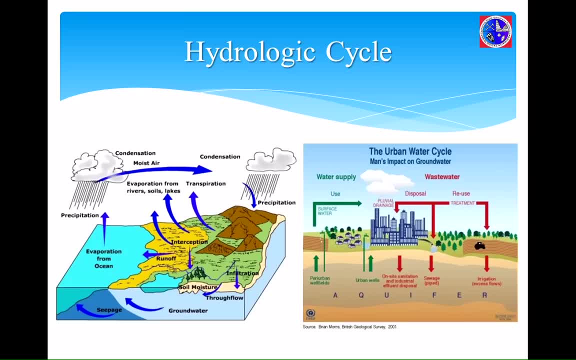 She went up to some friends- We were on vacation- It was last week- And she goes. you know that water you're drinking was dinosaur pee. you know All water on Earth is recycled, you know. And just here's another nice little picture I like from the USGS. 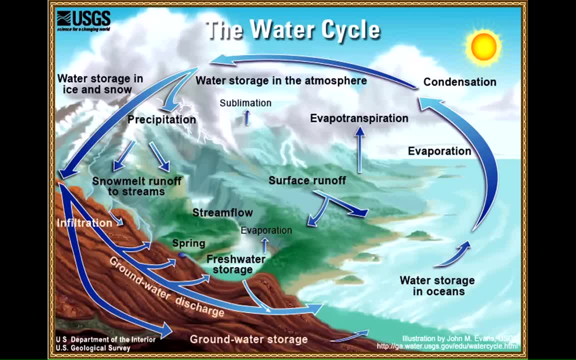 talking about the water cycle. It gives us a few other terms in there, nothing we're too worried about. Certainly there's storage, but groundwater is the one we're worried about And there again, you know when you pull it out and use it and put it back in. 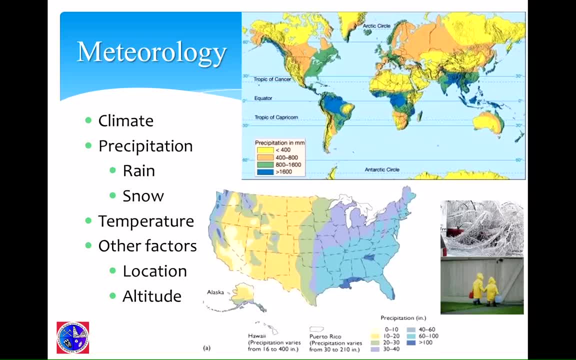 you're just keeping the system going. Why give it to the ocean? So, meteorology, why would I talk about that? Well, remember, in our water cycle, it's the first step, right? So we have to talk about climate. 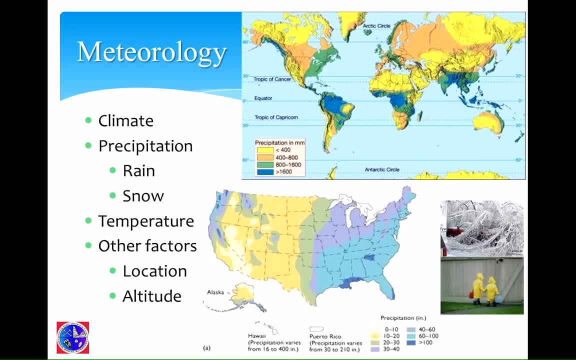 Lots of things out there with climate change, global warming, all these things. Is it true or not? I know my audience. I'm not going to sit here and say global warming. Climate's changed, though. 12,000 years ago, Chicago had a one-mile thick sheet of ice on top of it. 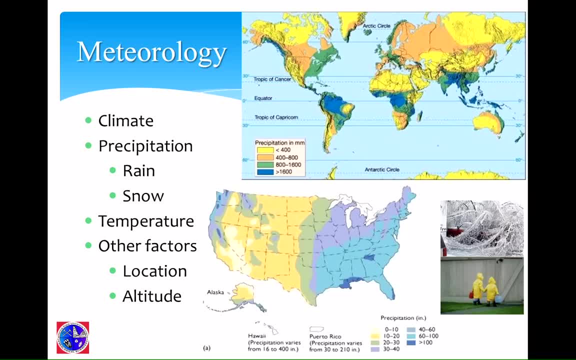 A mile thick. Is it there today? Anybody been to Chicago lately January? it feels like it, but it's still not a mile thick. That was 12,500 years ago. Were there a lot of cars driving around coal-fired power plants? 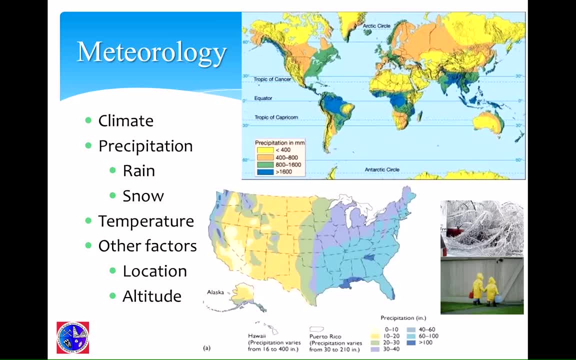 No, Climates change, They warm up. Now what the impact, the human impact, is on that, I don't know. There again, educate yourself and get your own opinion, But it does change And so it's going to change. 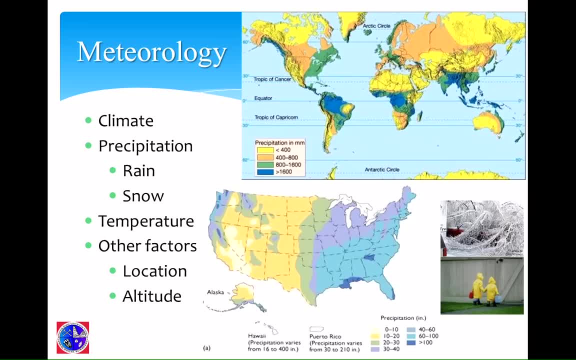 It has changed in the past and will change in the future. Temperatures impact, groundwater resources. Notice, this big yellow area is in the west and we don't have a whole hell of a lot of water- Lots of water- over here. Other factors is location and altitude and latitude. 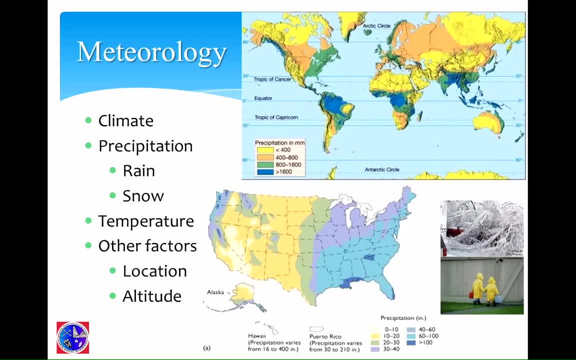 But all of that precipitation dictates what kind of groundwater resources we have. If you don't have a lot of precipitation, you don't have a lot of recharge and therefore you're limited in your groundwater supply. The other thing that's important- and I bring this up mainly because of the west coast- 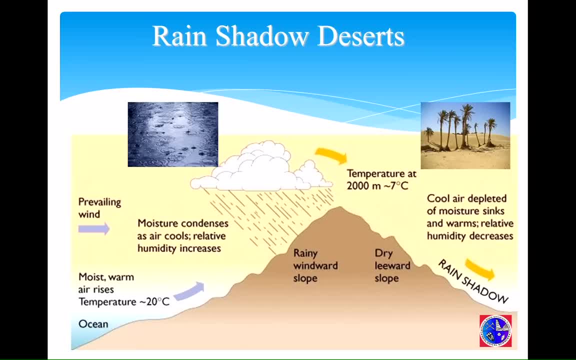 not so important for you guys is the rain shadow effect. As I tell my students, the Pacific Ocean, largest water body on Earth, lots of evaporation. What direction do the weather systems usually go in the United States? From west to east. 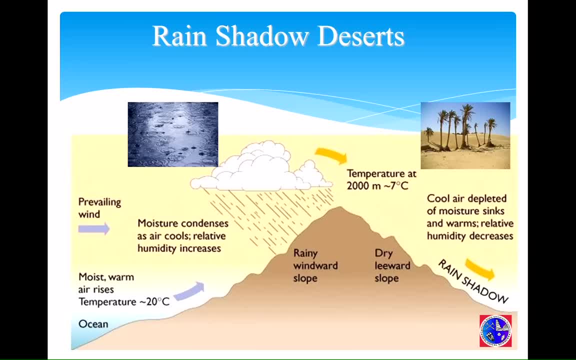 What happens? that evaporation goes up, the condensation happens, but that cloud is really heavy, It's got a lot of water in it, So it hits that first bump, which in our case is the San Bernardino or San Gabriel, but it could be the Cascades or the Rockies. 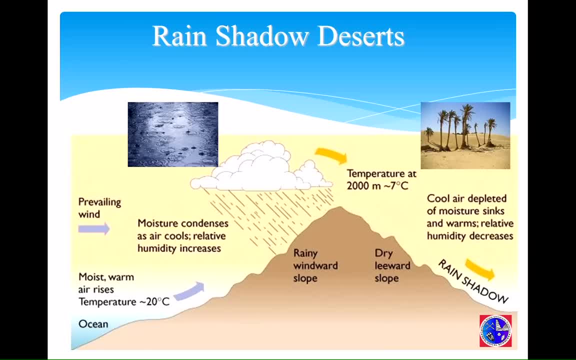 And what happens is that cloud can't get over the hill, So it precipitates out rains, snows, lightens its load until it gets high enough that it can float over. So we end up with this area on the back side, which gets less rain. 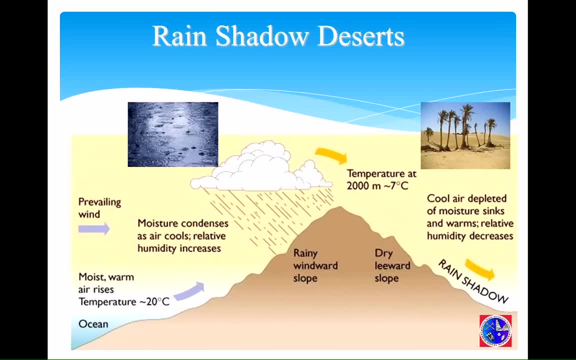 So you end up with a desert-type environment. The Mojave Desert would be a great example, But also Nebraska, and the Midwest through the Rockies has a rain shadow effect. So on the one side they get lots of rainfall, Very little on the other side. 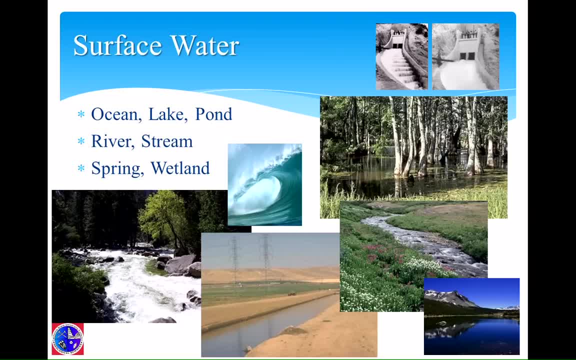 So surface water. There again, we can talk about it in all kinds of different fashions, from swamps to rivers, to oceans, aqueducts like we have in California, nice pretty lakes, But nonetheless it's a way for the water to move over. 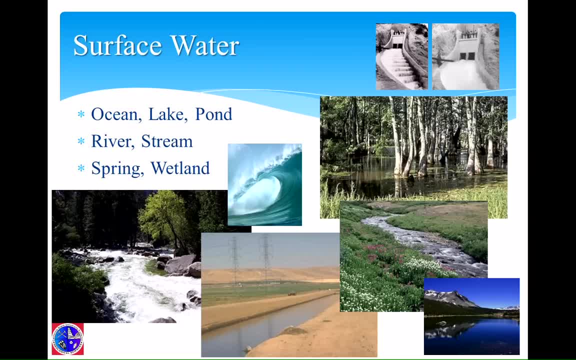 Now it's always touching the ground, So it can be a gaining stream or a losing stream. What do I mean by that? Certain locations along that water pathway, the water is actually going into the ground. It's losing: 100 gallons come in, it's only 50 go out. 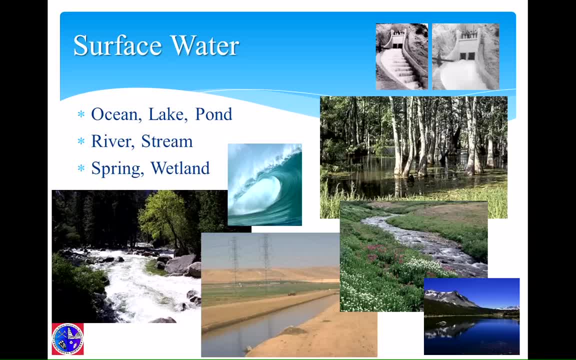 Where do the other 50 go? Into the ground? Other places that water is coming in. It's a gaining stream. How do you know the difference? by looking at them? Does that stream flow year-round? Why is there water in that river and it hasn't rained in months? 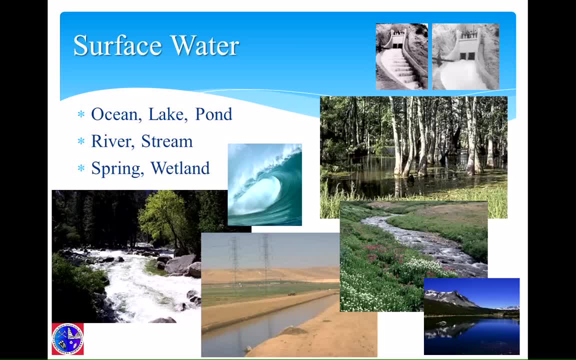 That's because groundwater is discharging into that creek or stream, allowing it to keep flowing, Where, if you go to the Mojave River, it's a river with no water, Because when it does, rain water goes along it for a ways. 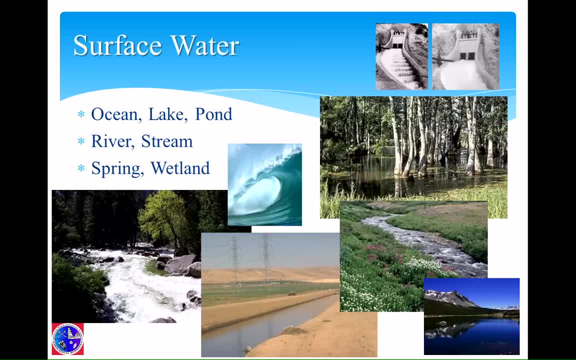 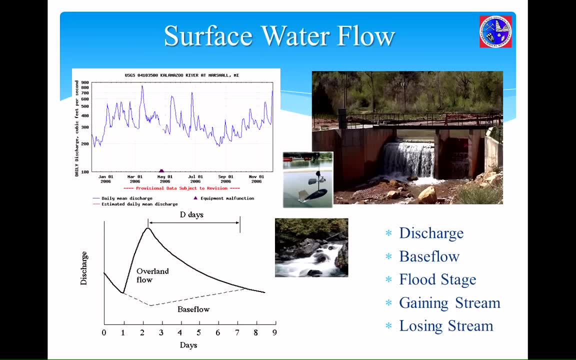 but it's always going to the ground because the groundwater is about 900 feet below it. So in the Midwest you don't have to worry about that so much, but us West Coast people do. And the way we study surface water is we look at what's called a hydrograph. 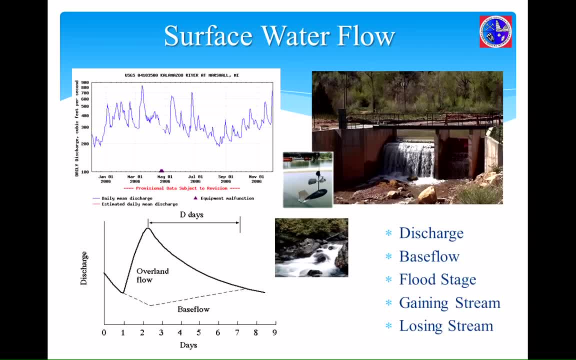 which is really time versus discharge. So here maybe a rainstorm happened and we get a little bit more water in the river and it gets dry for a while. So you can kind of look at things over time And what happens is, you know, water is going down and we get this big peak. 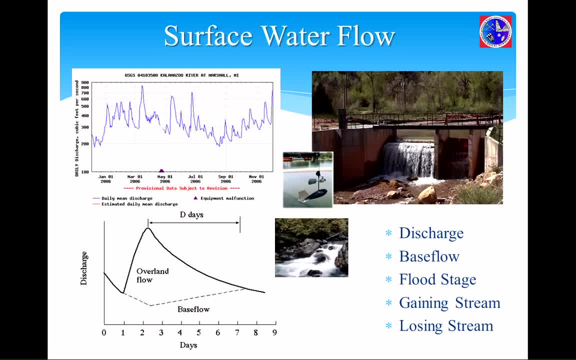 because the rainfall happened. then over time it dissipates. Well, if you can imagine, when water hits certain parts of the watershed, it takes a while for it to get to the river, And so that tail gets drawn out. Now from planners and engineers. they're always trying to figure out how to take this peak. 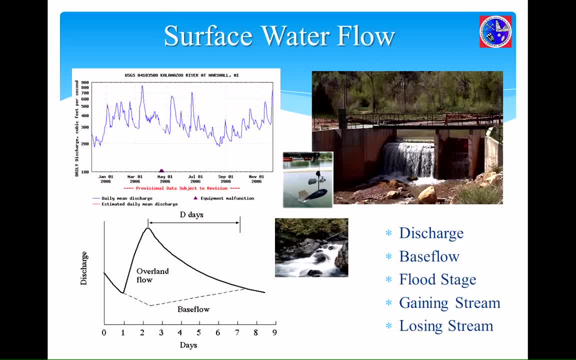 and knock it down, because that peak is what causes mass flooding. Okay, In certain areas. that's why we have flat rooftops on big buildings. They actually want to store some of the water up there so it doesn't hit all the storm sewers or storm drains at the same time. 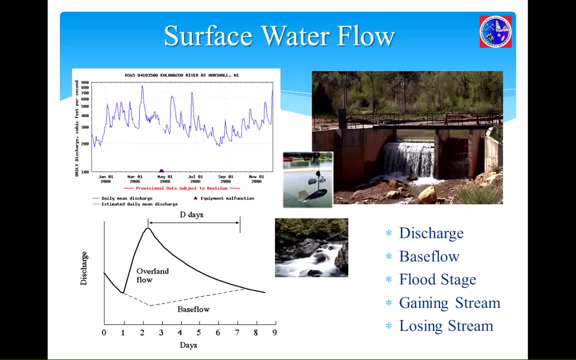 Because if all that water went to the storm drain you can't make a big enough pipe for that flow. So in order to do that, they store the water temporarily and then kind of discharge it over time to those surface water bodies, And so here's a nice illustration showing a gaining stream there. 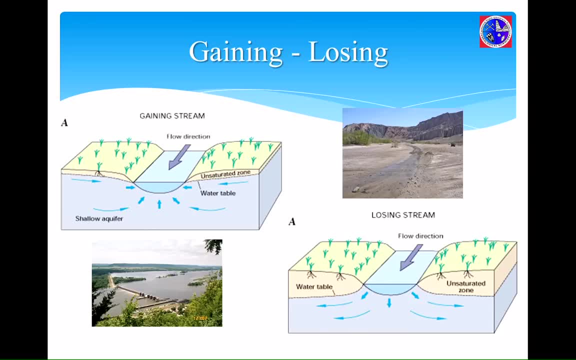 Again, groundwater is feeding that surface water body. This could be a lake or a stream or a river. It doesn't have to be just a stream, But groundwater is actually coming into it and discharging and then flowing over And other times where the river is actually higher or the lake is higher than the groundwater, 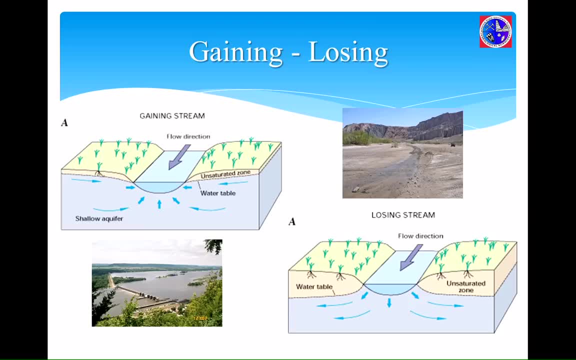 and you see it going out. What's interesting and what I never thought of was: this is great. This is book stuff, right, But the Mississippi River has places along it where it's gaining and places where it's losing, So it doesn't always have to be the same for every inch of it. 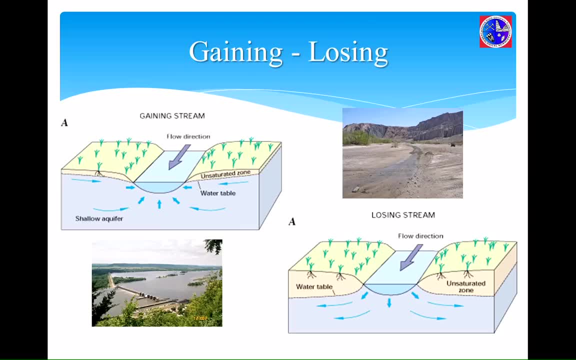 In fact, one of the things I did for my dissertation was look at the Kalamazoo River in Michigan. There, over a stretch of 50 feet, it switched to 100%, where it was 100% gaining, to 100% losing, over a 100-foot stretch. 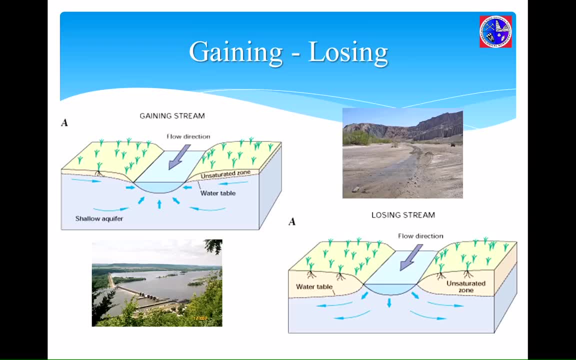 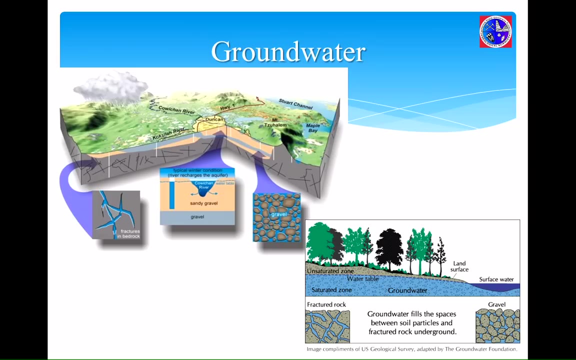 And it did that at different levels down the thing. So it can be really short-lived, But nonetheless it's that interaction between that surface water body and the groundwater which we're really talking about. So let's talk about groundwater, That's the water that's in the soils or in the rock. 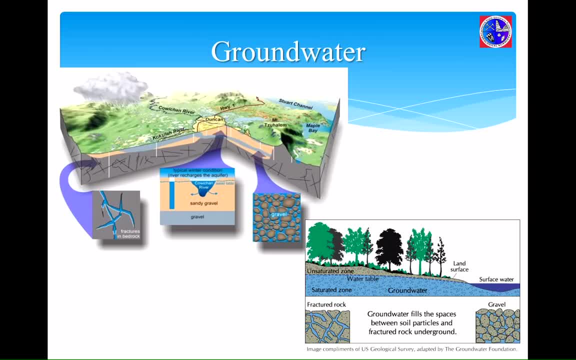 It's the stuff that sits in between all these fractures and these grains. It's stuff that we can't see. What I love about groundwater and love about teaching about it is: you can't see it, So I'm always right. You can't prove me wrong. 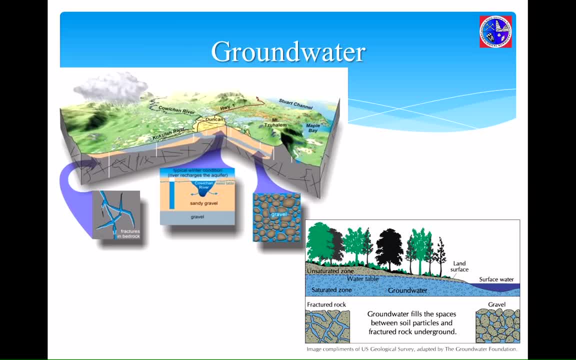 Surface water. any monkey can teach that stuff, because you can go out and touch it. You can't touch groundwater unless you do something with it. That's either go to a spring or put a well in the ground. Okay, What is it? 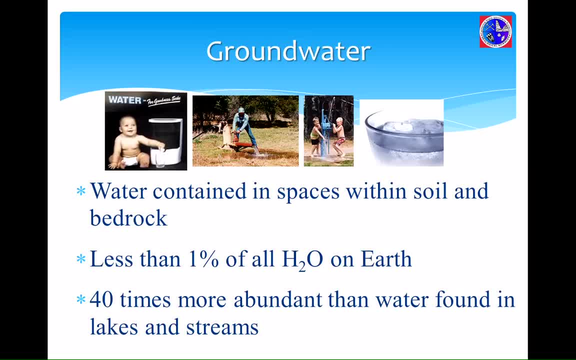 It's the water contained in spaces within soil and bedrock. It's less than only 1% of all water on Earth, But it's 40 times more abundant than lakes and streams. That's the key: The groundwater, even though it's minimal. 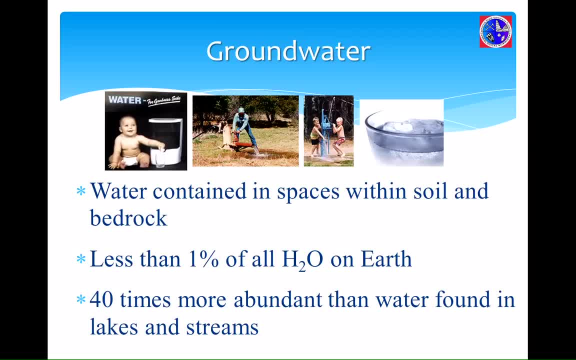 it's still so much bigger than all that fresh water that everyone thinks the surface is great And our politicians can vote on big river projects because they can see it. It's tough to vote on a big groundwater project because you can't see it. 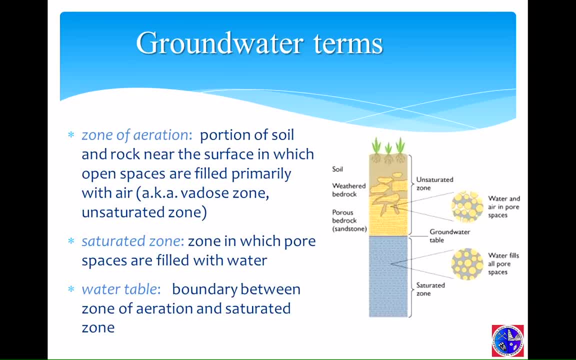 So some other terms: Zone of aeration, or vadozone, or unsaturated zone. That's the zone from what we walk on down to some level which I'm going to call the water table. At that point, everything is 100% saturated with water. 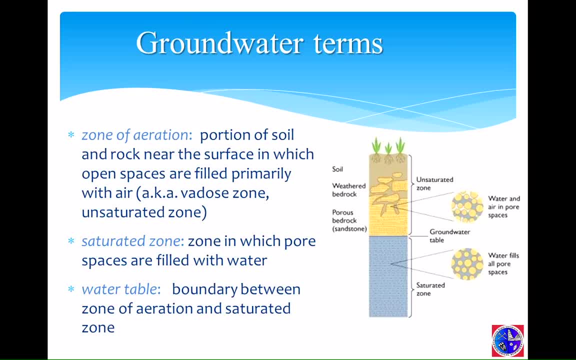 So all the void spaces in between the fractures and the sand, grains or clay or whatever else. it has water in it. Above that water table is what the vadozone is, And in here we can have water, but we also have air. 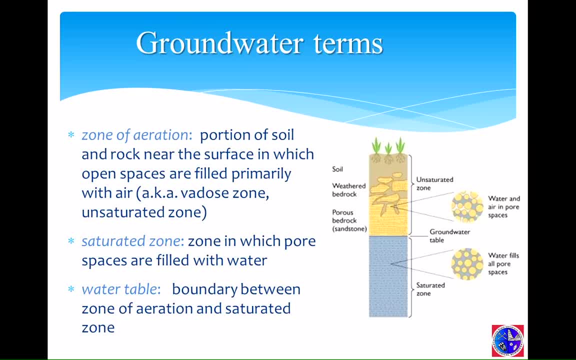 It's not 100% saturated And it has to have some water because the water had to get from here down. So those are some terms. So we have this as a vadozone, or unsaturated zone. Down here we have my aquifer. 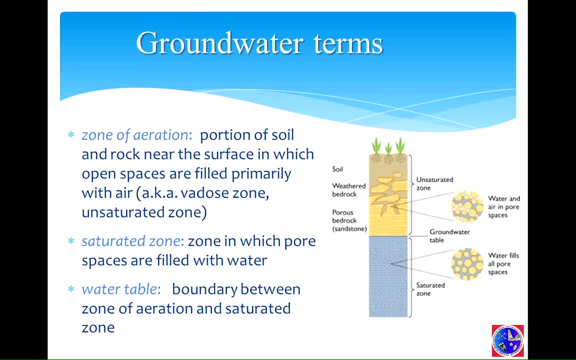 And that's the saturated zone, because everything is filled 100% with water, And the water table is the boundary between them. Now, what makes it complex is this is what's called an unconfined aquifer. So if I was to just dig a well, 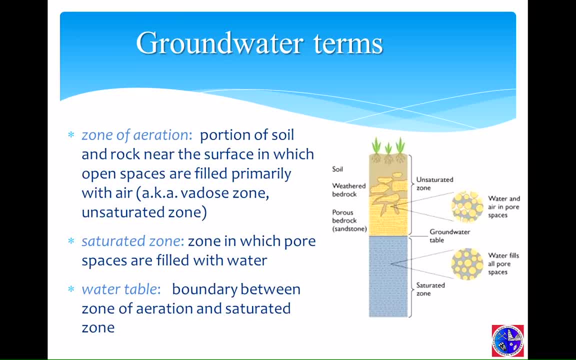 there's no clay in there, there's just sand. go down my sandbox, I hit the water table. it's pretty easy to recognize. It's also for those of you who dig in sand and gravels. it's right where the hole starts collapsing on you. 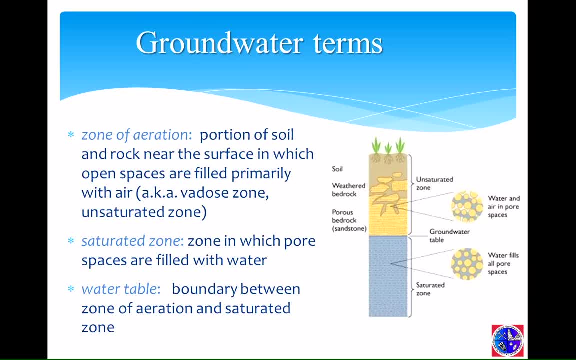 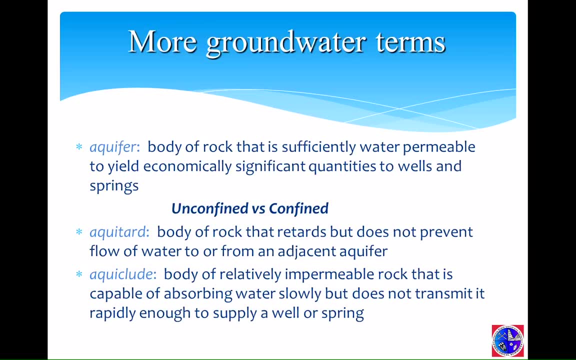 Because from that point on, the pressure is into my hole, not out of it. Above it, I can keep the hole open just by digging a hole. So what is an aquifer? Well, that's one. this is a definition. 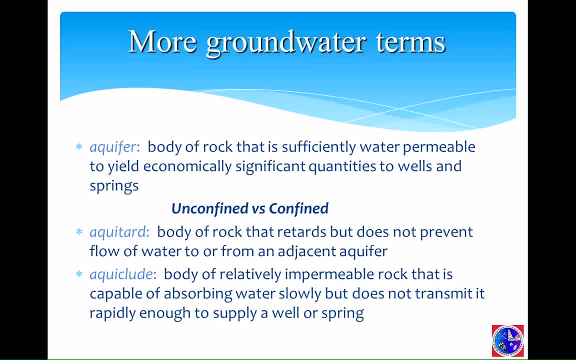 not necessarily the best one, but it's a body of rock that's sufficiently water permeable to yield economical, significant quantities of water to wells. What the hell is economical, I have no idea, because everybody's book is going to be different To me. the aquifer is that first body of water. 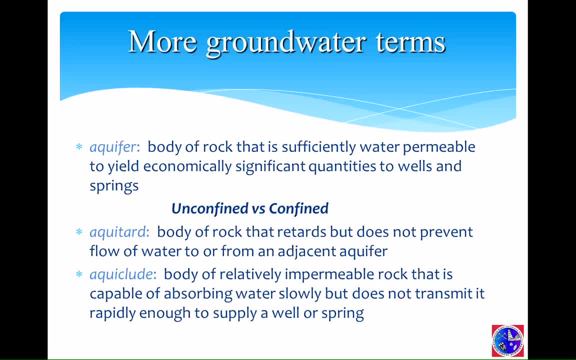 or first soil unit that's 100% saturated with water, regardless if it's rock or whatnot. The key is going to be this: unconfined and confined Now, and you've got karst around here, so it's probably an unconfined aquifer for the most part. 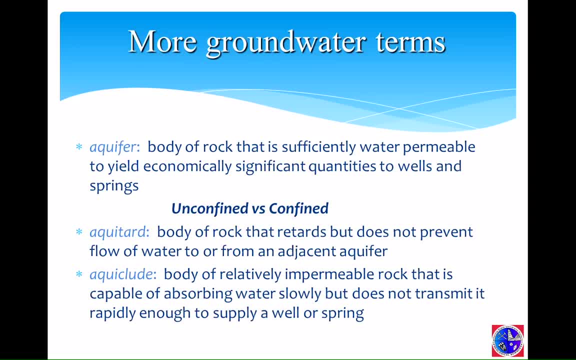 Is that right around here? I mean, does it go up and down with barometric pressure changes When it rains? do you see a response in your wells, Tennessee- I don't know Anybody here from Tennessee- At least one person brave enough to raise his hand. 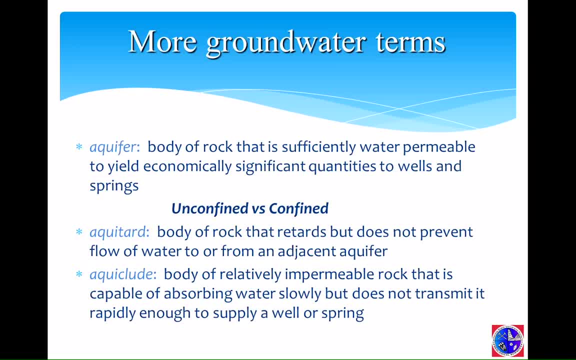 That's good. An unconfined or confined. Unconfined to me means that when water hits the land surface it can go unimpeded down to some depth. at that water table There's nothing to slow it down, It goes straight there. 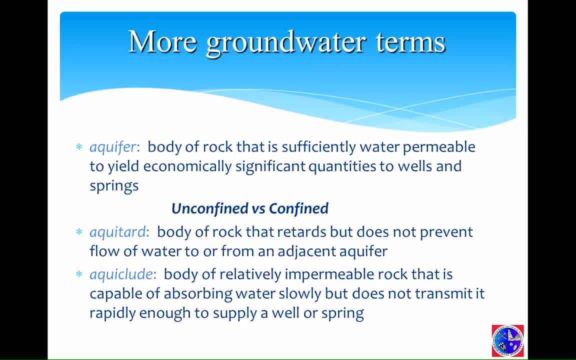 It also means when you have a weather system come through and the barometric pressure changes, I can actually see the water level go up and down based upon that pressure system. A confined aquifer is just that It has some rock or clay unit that is semi-permeable or impermeable. 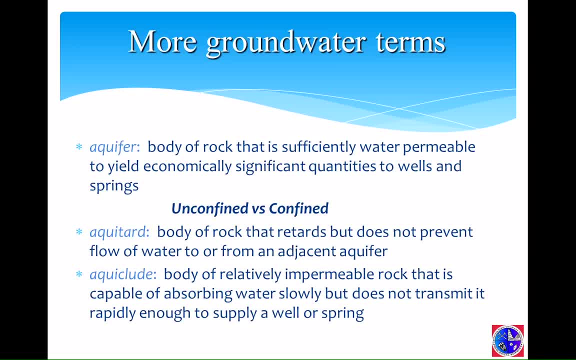 sitting on top of it, allowing pressure to build up below that, And so when it rains, the water doesn't get there directly. It has to go somewhere else, maybe recharge from a distance away, And so I'm going to show you a picture here. 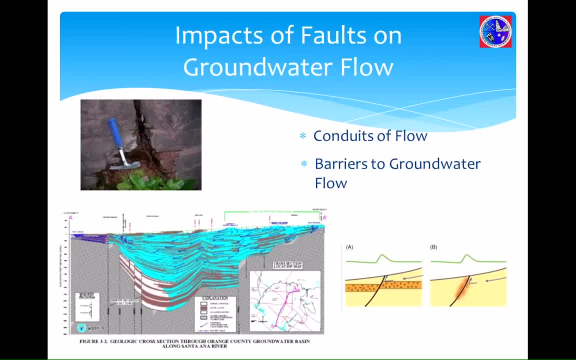 and hopefully we can talk about that a little more. Well, here's another one. You guys don't have a lot of faults around here, do you? Okay, anybody from Tennessee, Is there any faults around here? Okay, then there are some faults. 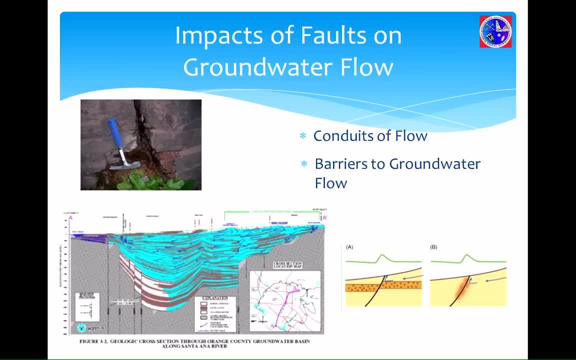 But they can be a conjunctivitis, a fluid for flow or a barrier to flow, depending on what they are, And this is some research we've been doing. Some of the rock units we're finding the faults are actually acting as rivers. 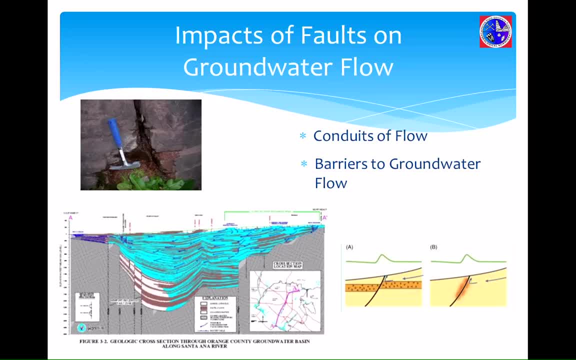 underground rivers, as much as I hate that term. But here's a picture of Orange County's aquifer. Each of these brown things represent confining units that are pressurizing or allowing the water down to be pressurized. We have recharge up here that feeds this middle of this basin. 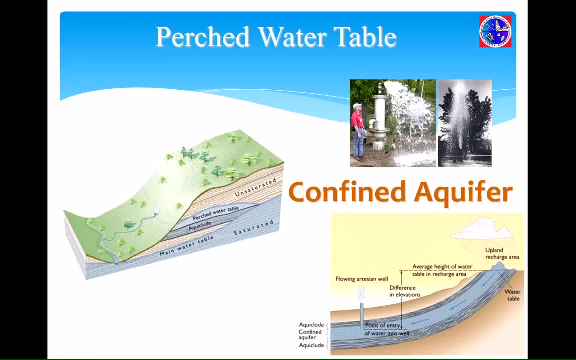 We'll talk a little more about that in a second. So a confined aquifer, as we see here, has a confining unit on it, has a rock unit that's not allowing water to perfectly move through it. Now, one of the things I always tell my students is: 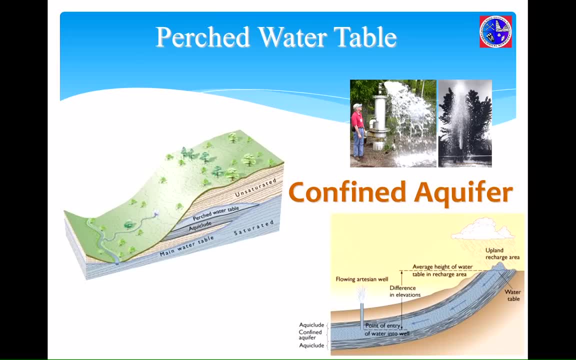 everything is permeable. Given enough time, water will find its way into anything and everything. That time is the question. So when we think about confining units, we're looking at something that takes hundreds of thousands of years to get through it. 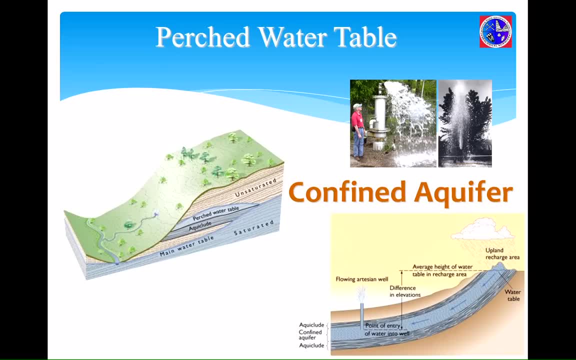 It'll get through it When you put water on this table. sooner or later it'll get through it, But how long will that take? You can actually have some perch systems as well here, where you have what's called an aquaclude or an aquitard. 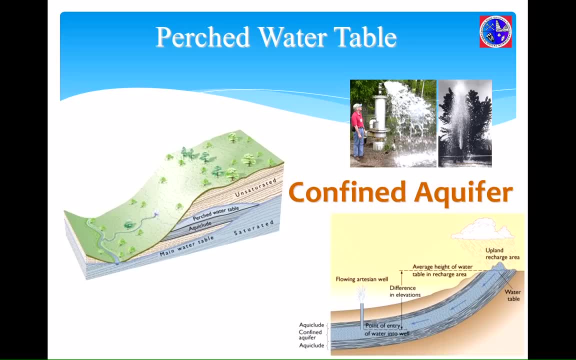 just different schematics for the same thing. But you can have water perched on top of it even though you have some beta zone down below it. So that's something that happens in the glacial areas quite a bit. I mean, we're finding all kinds of little thin silt units. 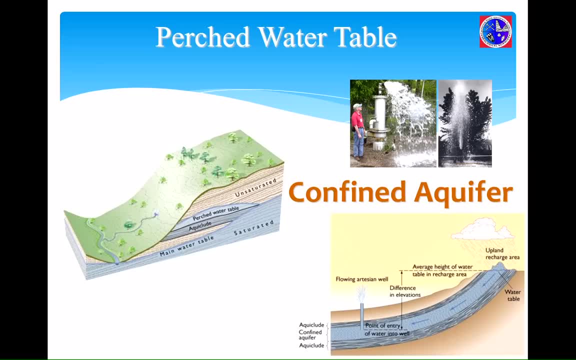 that are holding five or six feet of water. You drill through that. it's dry And for contaminant work that was really horrible, because you drilled that little one-inch layer pretty quickly And then all of a sudden it cross-contaminates something that wasn't contaminated before. 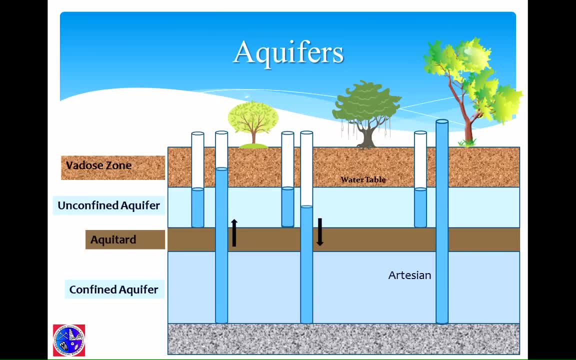 So here's my little scheme: A bunch of wells. Here's my beta zone, So in here I have both water and air, But then I have my water table. So this is an unconfined aquifer. It goes up and down with rainfall and barometric pressure changes. 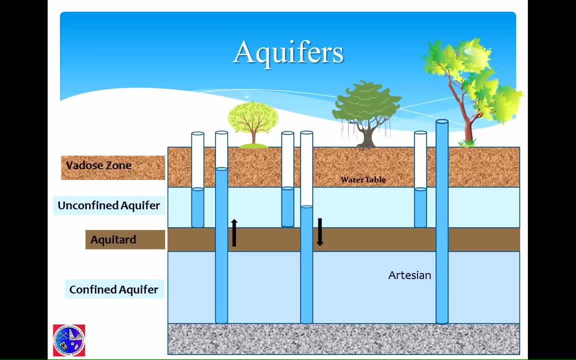 However, here I have a rock unit or a barrier to water moving across it, And down here I have another aquifer. Now, where'd this water come from? Probably from something off to the hills somewhere, But it's under pressure. 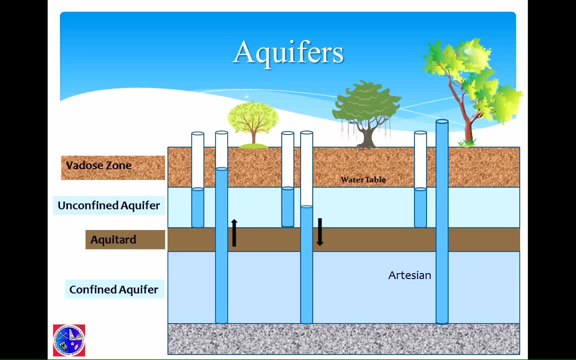 So how do I get an artesian? well, Well, when I drill into this thing, if that water level comes above the surface, we call it artesian. But where'd that pressure come from, That elevation for which the water will rise here? 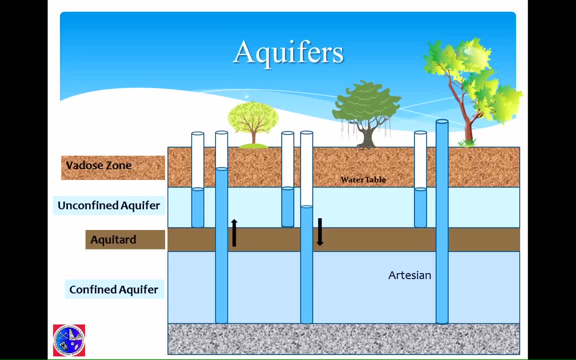 is equal to whatever the recharge elevation was at some distance away. Does that make sense? It's up in the hills. That's why you can get water flowing nicely. These are the kind of wells everyone likes to do, One of the things I want to point out here. 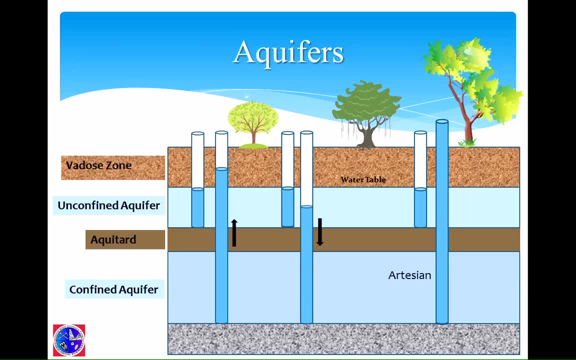 is that the water in this well, which is screened down here, is higher than the water in this unconfined aquifer, than the pressure is upward. Water moves from high pressure to low pressure, So this means this aquifer is pretty well protected. 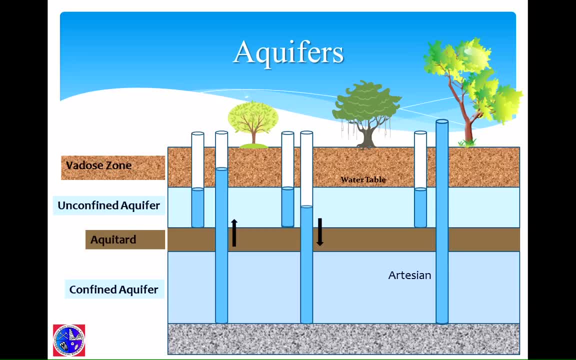 because its pressure is out of it, not into it. Where this one? since the water level is lower in this one than this one. the vertical gradient is downward, so this could be a potential aquifer for contamination transfer. So that's one reason why. 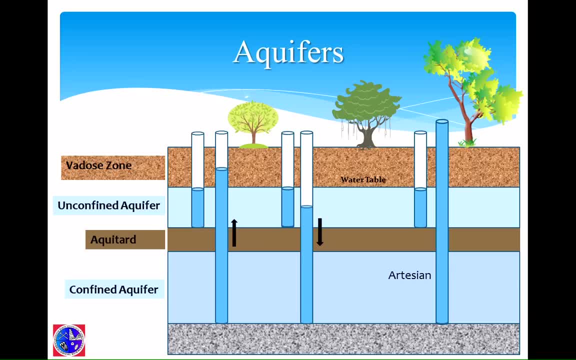 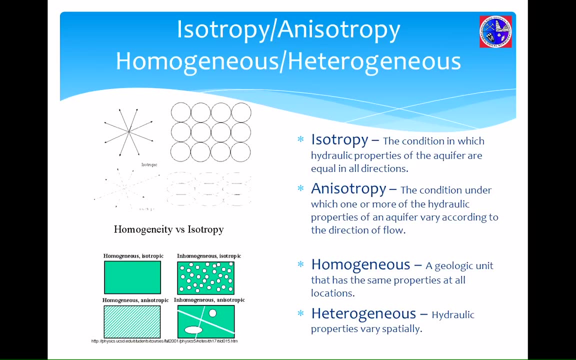 if you're ever doing environmental work, we put in nested wells. What do I mean by nested wells? Two wells next to each other but screened at different depths. We want to know if the water is moving downward or upward- Some other big words that we use in hydrogeology. 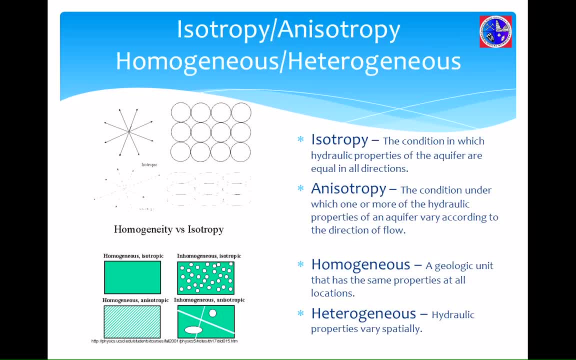 homogeneous and heterogeneous. Homogeneous means it's all the same in all locations, So beach sand is nice for properties of geology. Heterogeneous is going to be the clay or glacial outwash that has all kinds of stuff in it, And then there's isotropic and anisotropic. 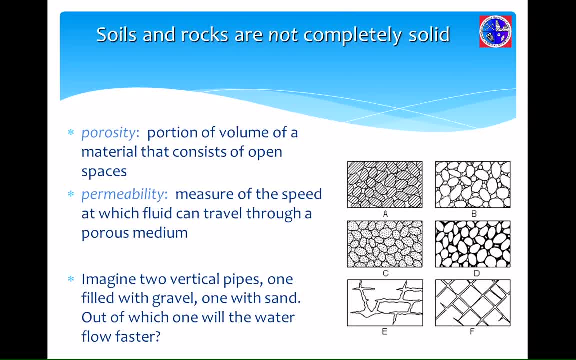 that we can talk about later. So what's that mean? for when I was drilling, it meant porosity and permeability. And what's the difference? Porosity is that number we give to the volume of water a soil can hold. Permeability is 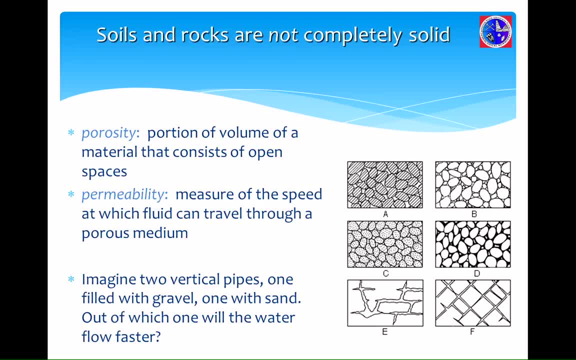 can that water move through that soil? So one of the things I always tell my students is: what's the porosity of sand versus porosity of clay? They're about the same. They hold about the same amount of water, Somewhere around 35 to 45%. 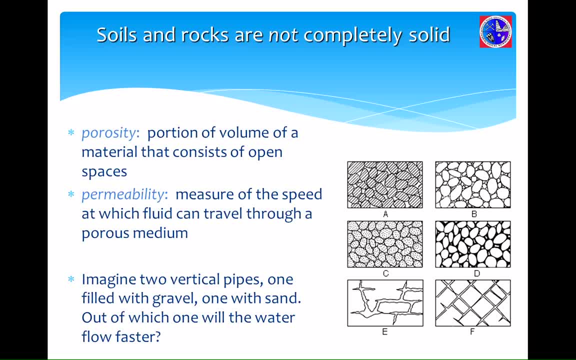 they can hold water. But permeability, which is what I really care about, is how that water moves through it. Clay is pretty low, Sand pretty good, So we get confused a lot of times by talking about the porosity of stuff. 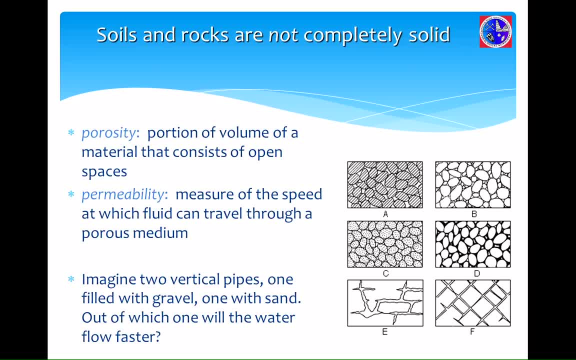 because it may be the same porosity value, but the permeability is what I really care about, because I need to get that water to my well. I want to know how it's moving through that aquifer, So permeability is probably a better verbiage to use. 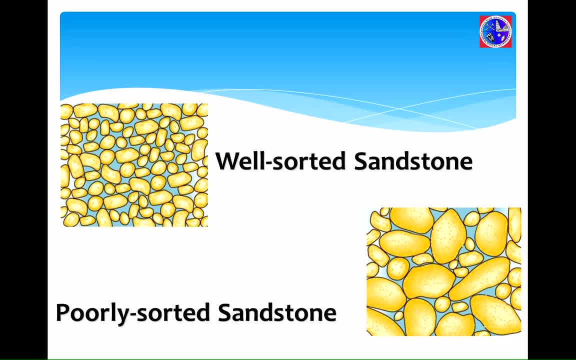 when we're trying to deal with water issues, Which brings me up to well sorted versus poorly sorted or well graded versus poorly graded. Now I did was the McElhaney Lecture in 2009,, so I don't know if any of you guys heard me. 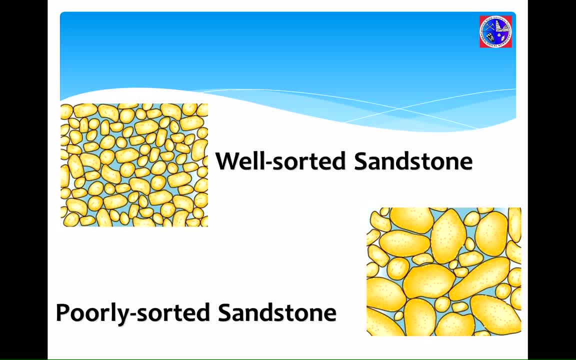 give my lecture on soil classification. Hopefully you did, and actually hopefully everyone is out there doing the unified soil classification system for the rocks and soils, right? No one has a clue what I'm talking about, right? That's good. I'm glad I spent 56 weeks of my life. 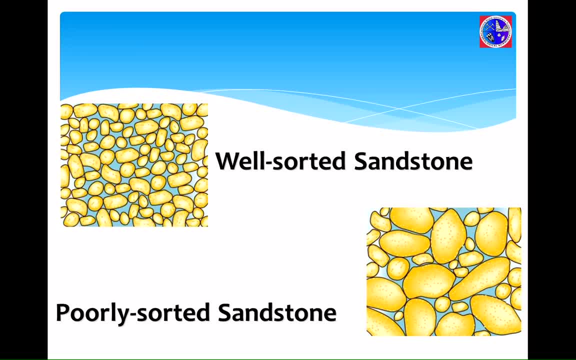 traveling the goddamn country and no one paid attention to me. Well, it's like the thousands of students I have that never listened to me either. Anyway, grading and sorting. We can relate this back to permeability. It goes to grain size. 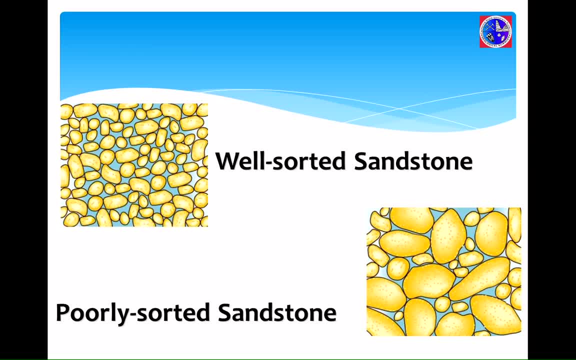 What I like to start with is grading. Grading means that I have- when I grade my class, I have a bunch of students get A's, some get B's, C's, D's and F's- A well graded class, according to the university. 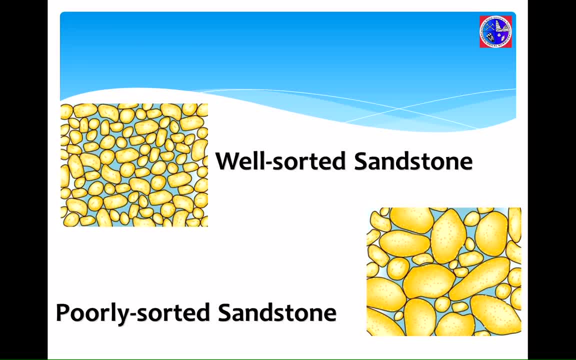 is I have equal numbers of grades for each of those categories. Poorly graded would be is I give my whole class a bunch of C's. So when we relate that to rocks, poorly graded means I have all one grain size. Well graded means I have some clay. 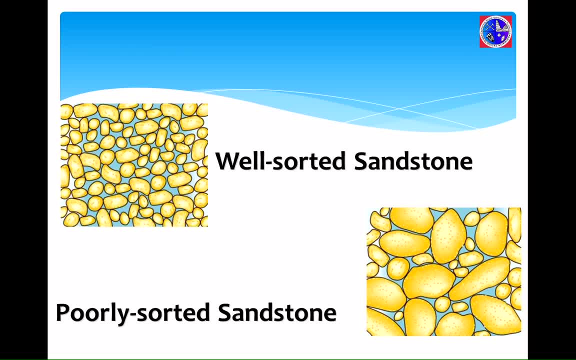 silt, sand, gravel and boulders. Sorting is opposite of grading, So if something is well graded, by definition it's poorly sorted. If it's poorly graded, it's well sorted. So just think of it as flip-flopping them. 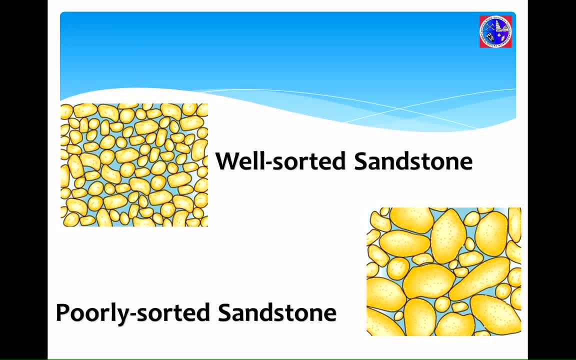 So in this case, what is this one? It's well sorted, so immediately it would be poorly graded. This one's poorly sorted, so it's well graded, And you can see I have a little bit of every different size. This one's all pretty uniform. 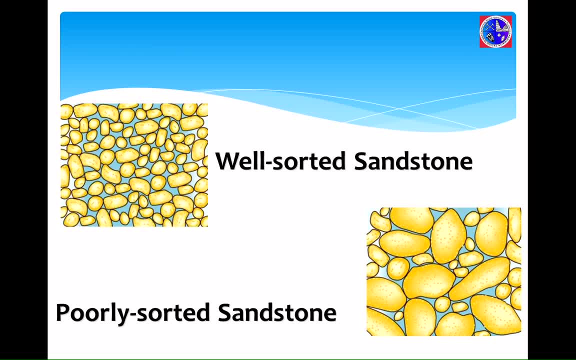 What's important about that is, from a water production standpoint or groundwater right, Which one is water going to move through easily? This one or this one? It's going to do this one right, Because everything's about the same. It's like putting a bunch of marbles together. 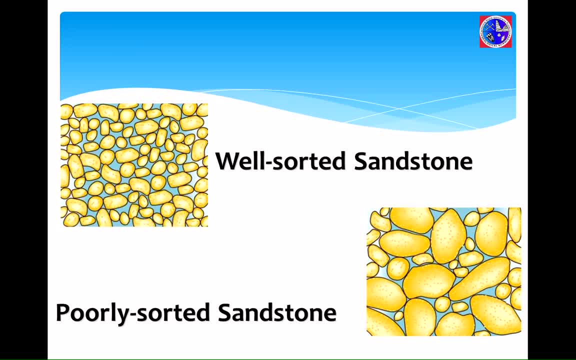 If I add BBs to my marble collection, it plugs up all those places for that water to go through, So it makes it more difficult. So from a permeability standpoint this has a much higher permeability than this guy does. So just because you find some gravel in there, 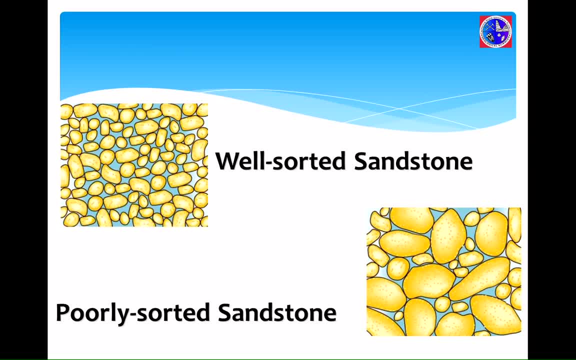 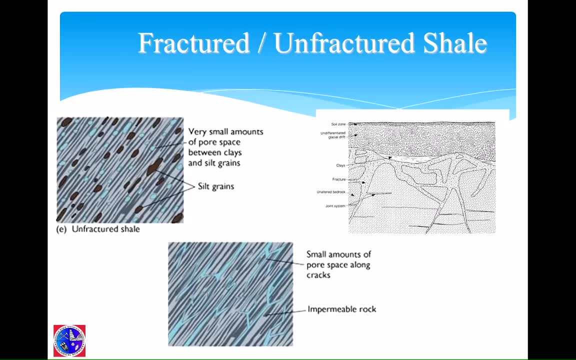 that may be great, but if there's a lot of clays and silts tied with it, that could be plugging up your aquifer, And the same thing can be happening with fractures, Okay, And curse systems. It's great that I have all kinds of large cracks down there. 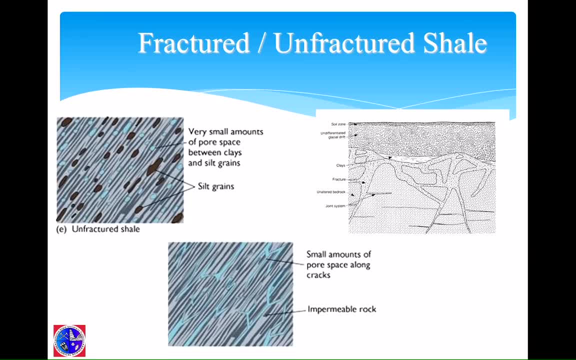 But if they're not connected to another crack, to another crack that ultimately connects to your? well, what good does it mean? It's great for storing water, because the porosity's high but the permeability is low. There's no connectivity between cracks and fractures. 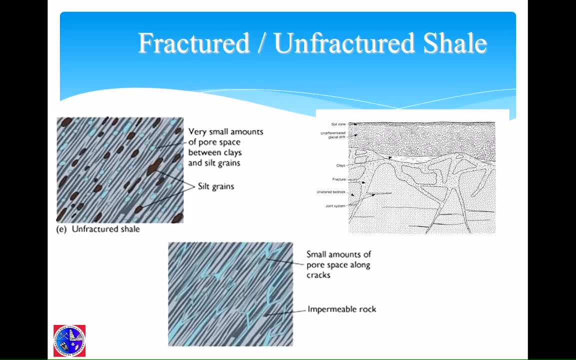 So it's that permeability or that connection between all those that's really important to us from a groundwater standpoint. Am I doing the time? Ah, plenty of time. We'll skip this one. Some of the ways we look at this and another term. you're going to hear a lot. 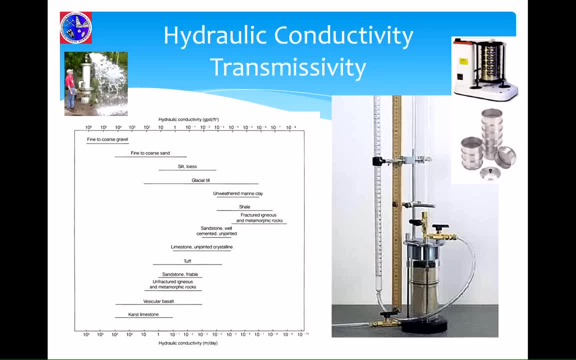 is hydraulic connectivity. Hydraulic connectivity, you think of that as permeability. It's the rate for which water can move through the rock media, And we have some different ways we can test that. We can sieve them. We have these little fancy permeambers. 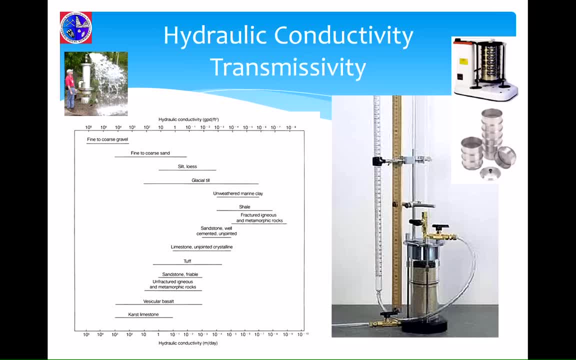 that you only see in the water, And then we can see how much water can move through the rock media, And we have some different ways we can test that. We can sieve them. We have these little fancy permeambers that you only see in the water. 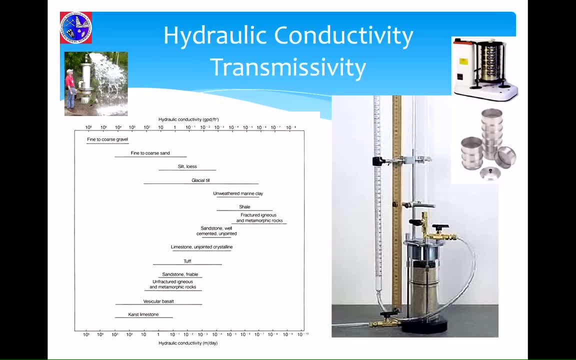 And then we can see how much water can move through the rock media And then we can test that We can sieve them. We have these little fancy permeambers that you only see in colleges. No one whose right mind would ever do it outside that. 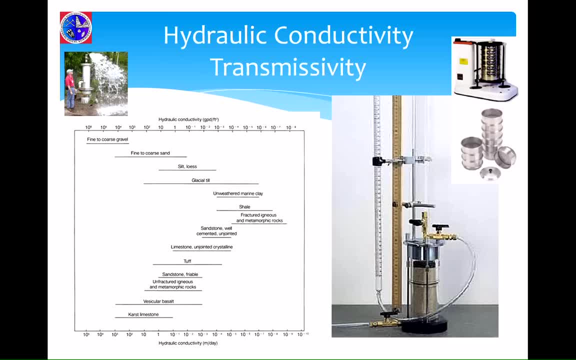 But this kind of gives us some idea of you know, there again shales are pretty low. karst limestone is pretty high. It can be up to several hundred feet per day. Down in Texas they did a study and they did some dyes. 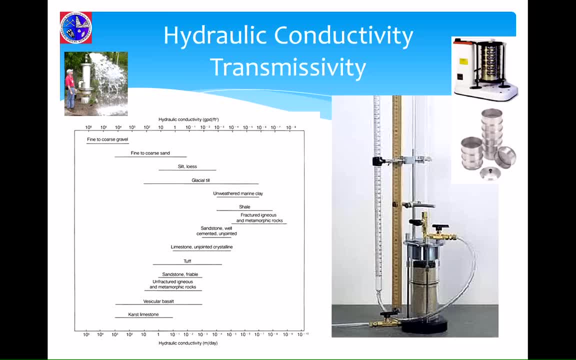 and they dropped them in one part of the aquifer, shot out about a mile and a half within two days. That's moving pretty quick. So you know, depending on what you're in, it can change that permeability slash hydraulic conductivity. 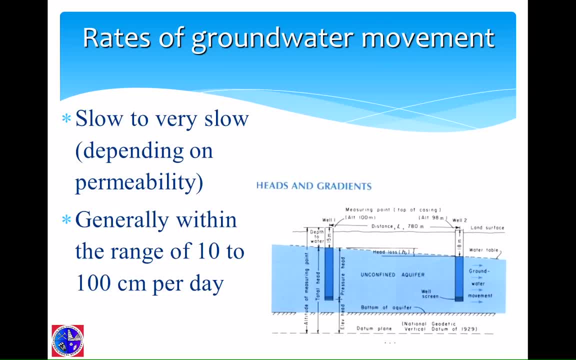 But for the most part groundwater moves pretty slow. It's not really a fast-moving system. Why? Because there – again it's on a tilt, And I'm going to show you that here in a second is it goes from high pressure. 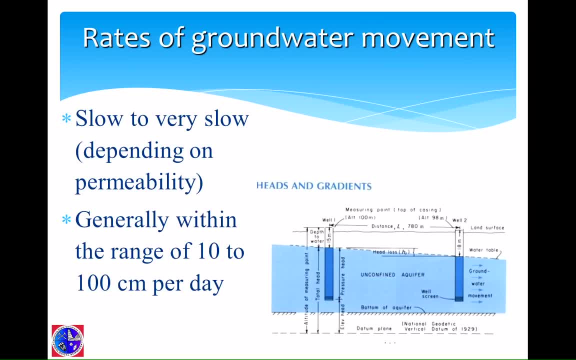 to low pressure And it has some – it has a bunch of rocks it's got to get through. So it's like you trying to get through a crowd at the airport: The bigger the crowd, the harder it is for you to get through it. 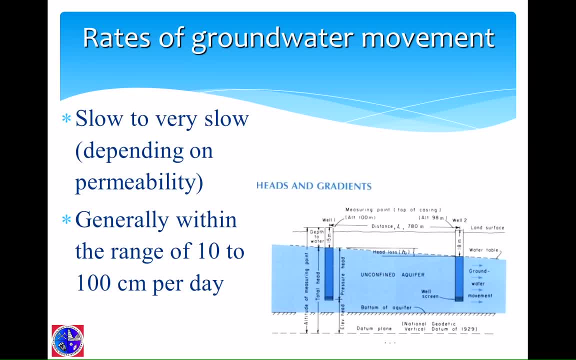 There's no one there, You fly right through Which, by the way –, how many people flew here this time? Did you have to go through the whole security thing Because they pulled me aside, which I thought, oh shit, Now I'm going to be strip searched for whatever reason you know. 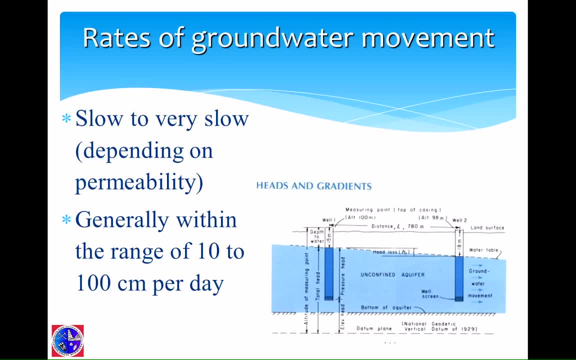 But no, I kept my shoes on my jackets, on my glasses, everything. They said there's no walk-through. My briefcase didn't have to take the laptop out. I was like, really, This is like the old days. 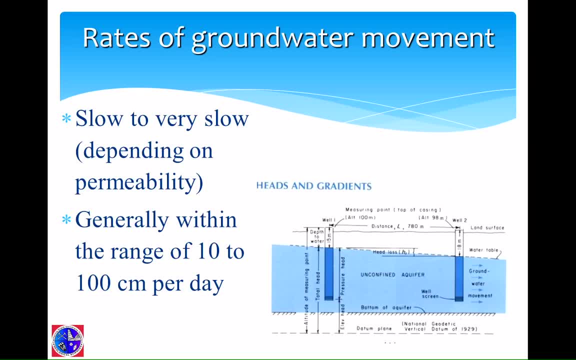 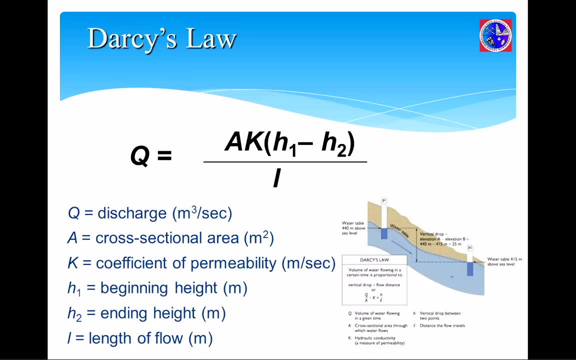 Oh, now on the way home, I'll get strip searched, of course, because it all evens out sooner or later. Yeah, So we have one law in groundwater. Now what is a law? Law of gravity? We've tested it enough times. 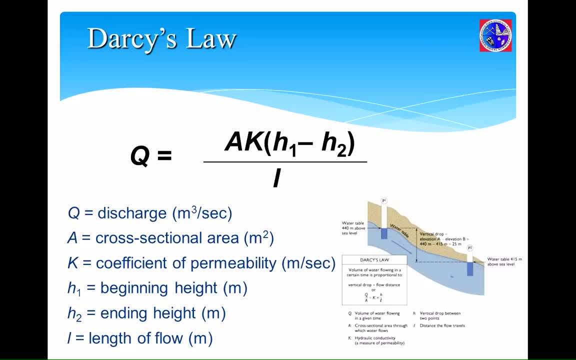 We've dropped the pencil, It falls down. This is our one law that we have in groundwater. It's called Darcy's Law, And it's a law that's really good in this case, And it's a law that's really good in this case. 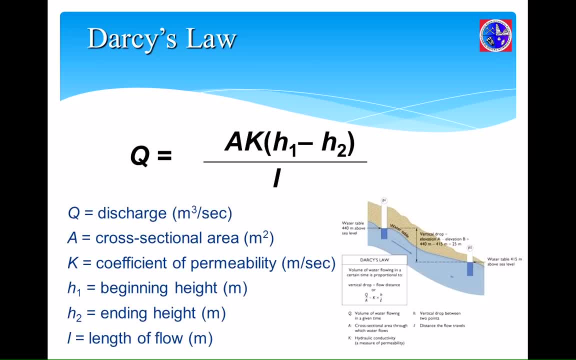 So I'm going to show you two things. I'm going to show you three things. I'm going to show you three things. I'm going to show you two things. One is this. The third is the number of blocks in this area. 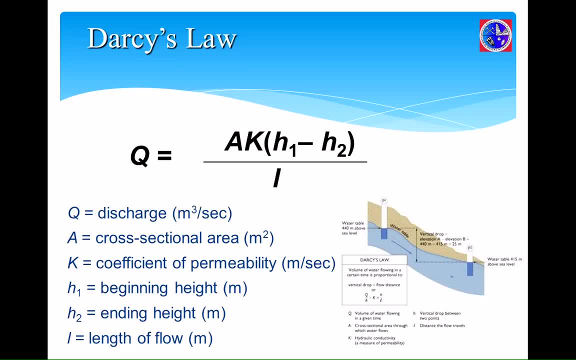 The fourth is the number of blocks in this area, And I'm going to show you three things So you don't panic too much about the giant equation. I throw this up here just so it scares the shit out of you and you have to hire me to. 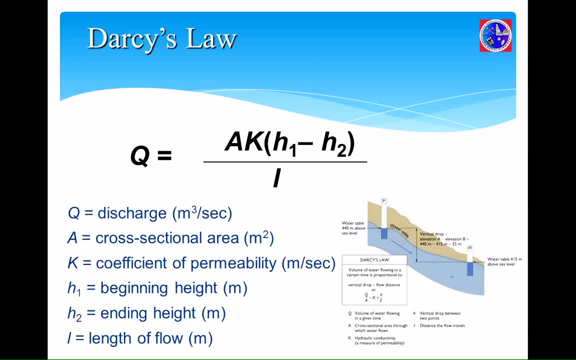 do whatever you need done. Okay, Really, what it is, it's my permeability number, this K hydraulic connectivity, The area that I have to move through, and my slope. You know what's the slope because it you know it's this height and that gives me discharge. 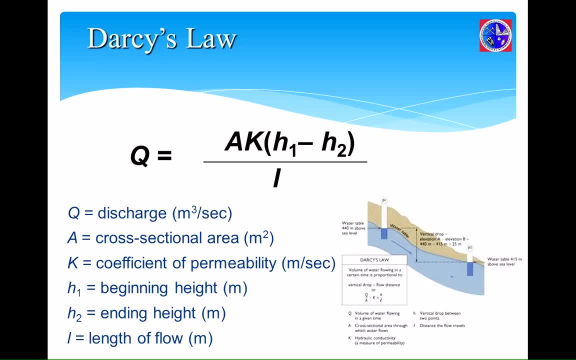 So now I can calculate how much water is moving through that aquifer, or how much water I'm going to get out of the aquifer, which is more important to most of us. okay, So by using this equation, we can calculate that. 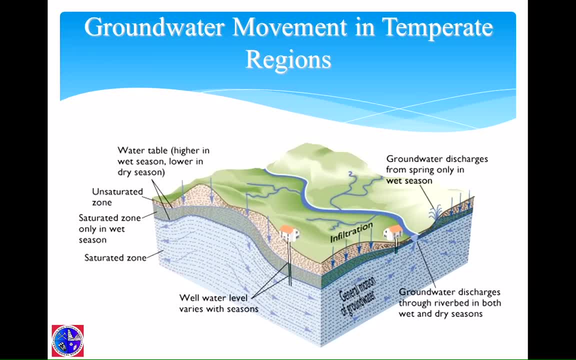 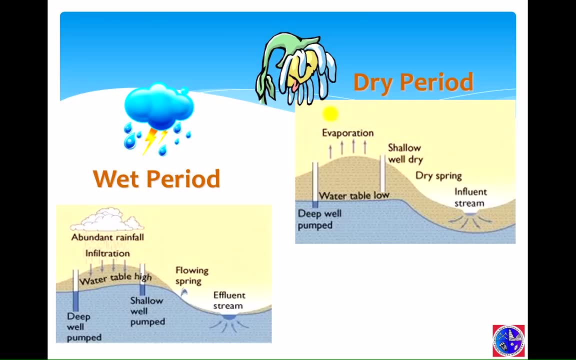 But groundwater moves differently in different regions. Around here it's car space, so you're going to have sinkholes and all kinds of disappearing rivers. Dry regions, as we'll see here, mean it could be, you know, wet and dry periods. 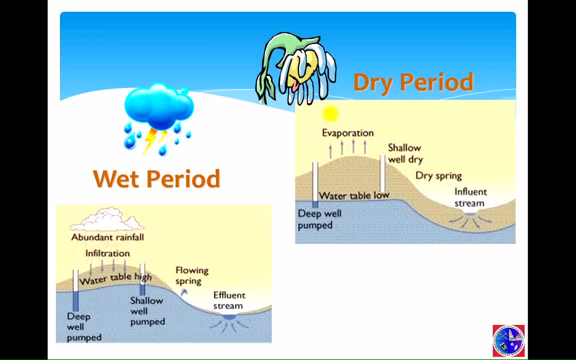 so water levels do go up and down, and so do the other things. So this all impacts our groundwater resources and changes with the times. This could be due to all kinds of different reasons, obviously. So it brings me to an equation which I think you guys can handle. 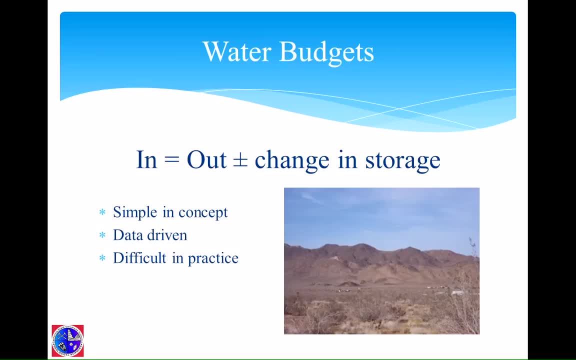 This is my favorite mathematical equation. It's called the water budget. okay, It's pretty simple. I have my glass of water. If I add water to my glass of water, what's the water level in my glass do? It goes up. 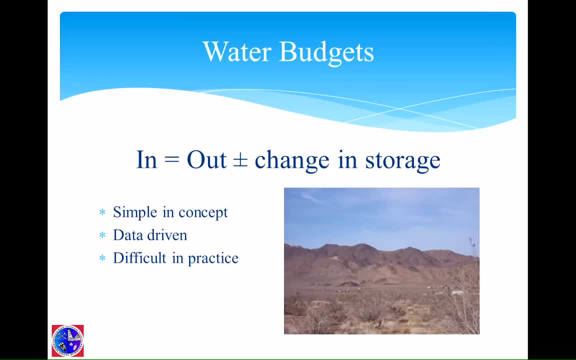 If I drink that water, what's the level in my water glass do? It goes down. That's – I can – this is my kind of math, okay, But it allows me to actually look at from a basin standpoint or a watershed standpoint. 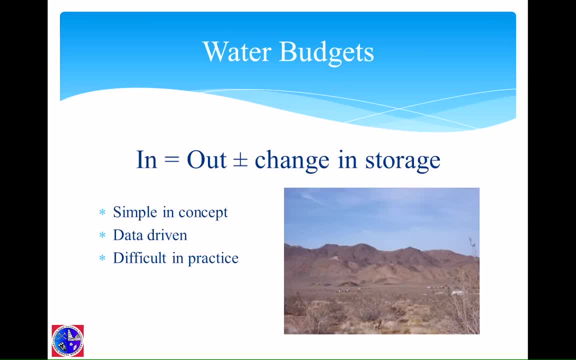 what's happening with my water resources? because it's pretty important, Because if I have more going in than I'm taking out – this is like your bank account- right, That's good. But if I start taking out more than is going in, what's that do to all the water resources? 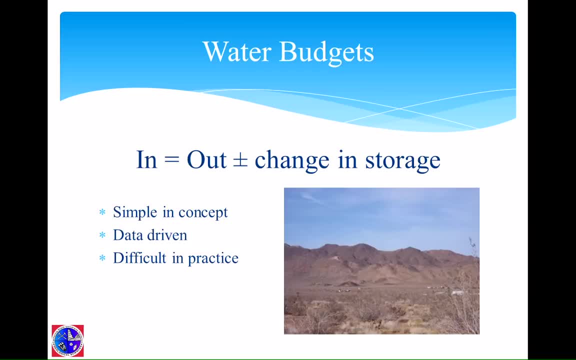 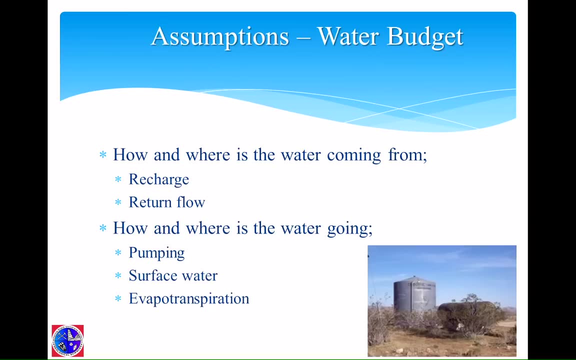 in that valley. They all go down. Okay, we're over-stretching and using more than we should, So it helps us become more sustainable, which is something we're all going to have to deal with as we move forward. So some assumptions we make is that we have to usually calculate what recharge is and 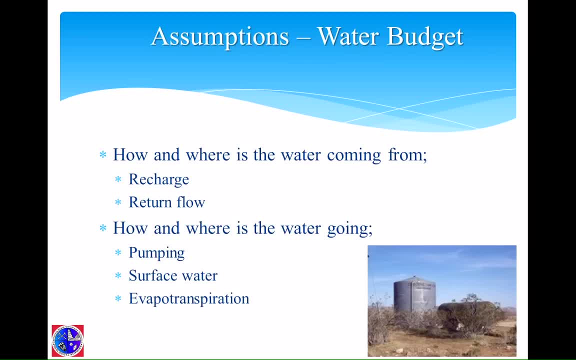 we usually look at rainfall. Of course, rainfall is sporadic. right, You can get rainfall in one county and none in the other county. So what does that mean? Well, it means you're getting rainwater, but the watershed, or my groundwater basin, may cover both counties. 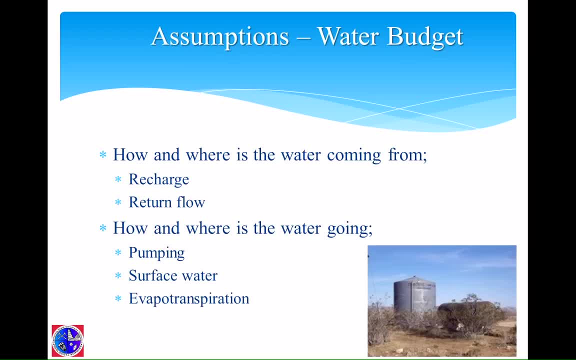 So you have to make some assumptions there: what the annual recharge might be. What's return flow? Anybody know- Anybody ever heard that term- How many people sit on a septic tank or have a septic tank at their house? Every time you flush a toilet, you're recharging the groundwater. 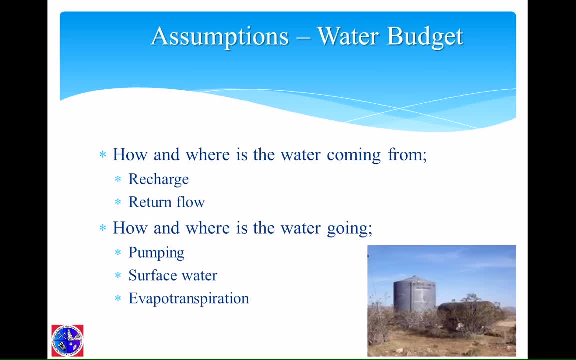 So we have to make some calculations with that And we have to make some assumptions. Other things we have to know is: what's the pumping going on in that area? And then surface water and this big evapotranspiration which is really the plant uptake. 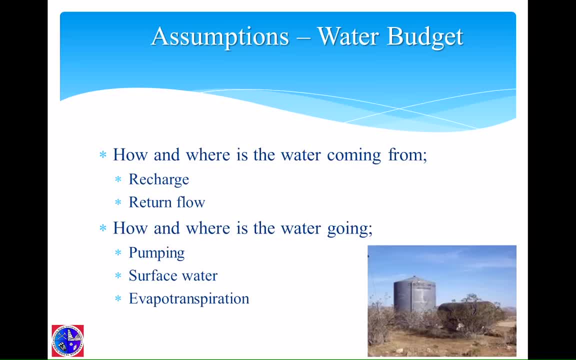 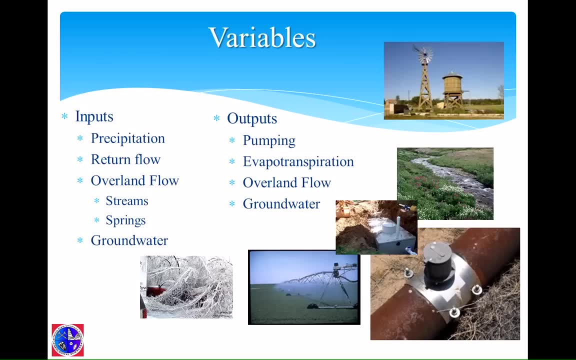 Plants steal water from us. Of course they give us some oxygen, which helps, but they do steal our water. So we basically line up our inputs and our outputs to our bathtub or glass of water. Our inputs are going to be rain and snow. 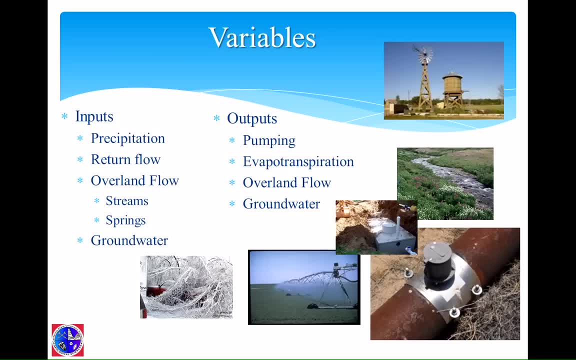 It's going to be that septic system that you discharge out the back. It's going to be some streams and springs coming in, But we can also have ground. We can also have groundwater coming into our area as well as leaving it, Because our outputs are our usage, our pumping plants, rivers leaving our area. 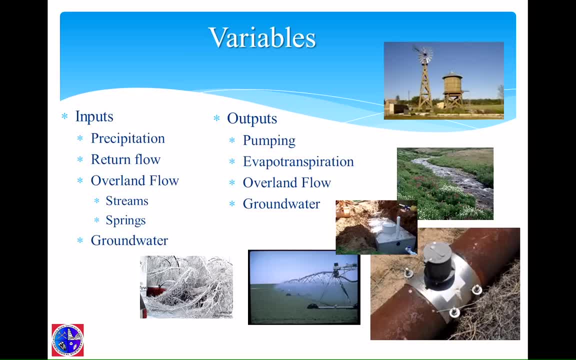 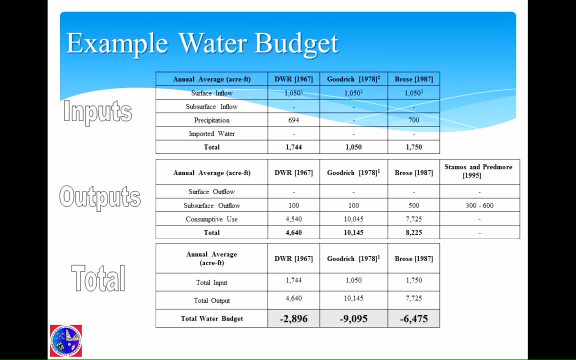 and then that groundwater leaving the area. Well, it's actually pretty simple to make these calculations, And so what I want to do is give you an example of one we did out in the Mojave Desert. some students of mine- I forgot their names already, so it doesn't matter. 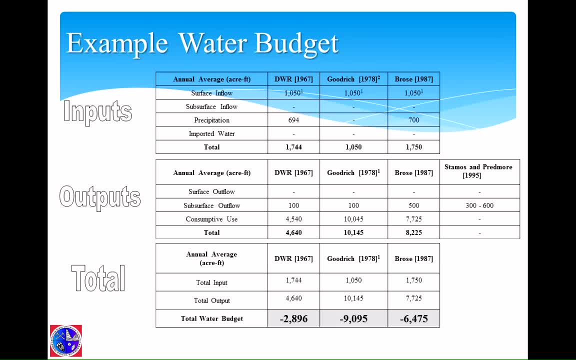 Here is our inputs. Here's three different people that did these inputs out there And these are in acre feet. It ranged from about 1,000 to 70.. 1,700 acre feet per year. end to my basin. The outputs were from 4,000 to 10,000 going out. 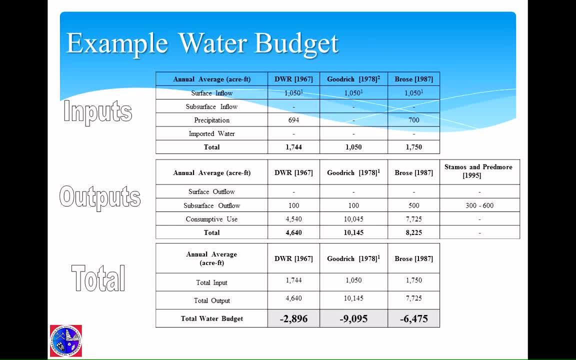 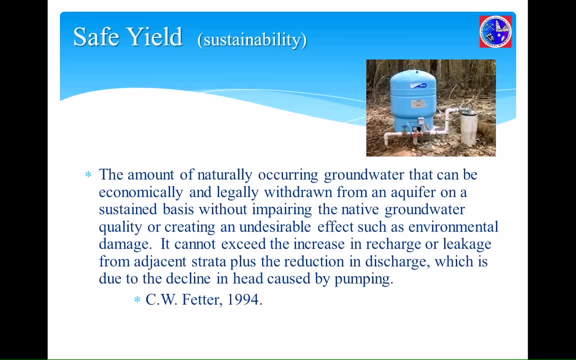 So what should the water levels in this basin be doing? Going down, And you see down here all these negative numbers. Well, let's look at safe yield. then I'll show you the hydrograph. This is straight out of a textbook. 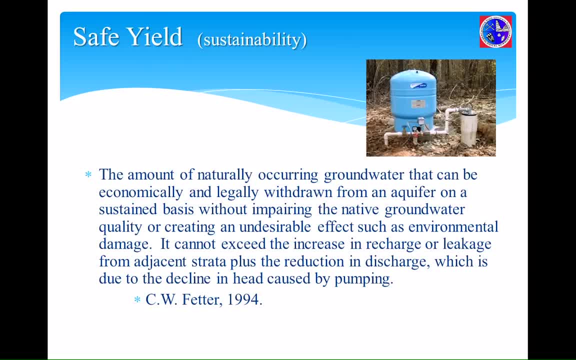 Safe yield is the amount of naturally occurring ground. It's the amount of groundwater that can be economically and legally- let me get the lawyers in there- withdrawn from an aquifer on a sustained basis without impairing native quality or environmental damage. So basically, what goes in should equal what's coming out. 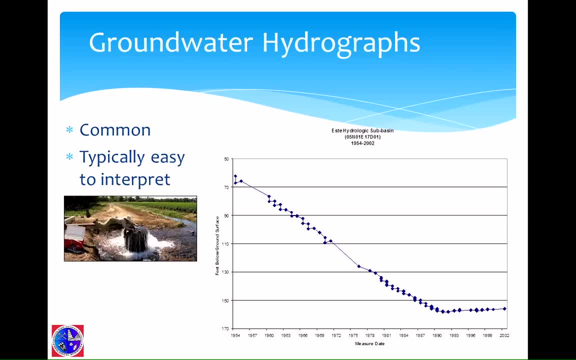 Here is that same hydrograph I showed you for surface water, but in groundwater. This is water levels taken in a well. Here's 1964.. Here's 1964. Here's 1999.. We're looking at about 80 feet. 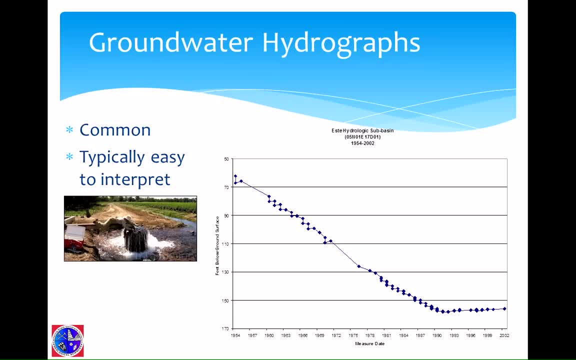 Not sustainable, You know, because sooner or later you're going to run out of water. But something happened here And we're going to talk about that, Okay. so with those hydrographs which we use in the hydrogeology field all the time, 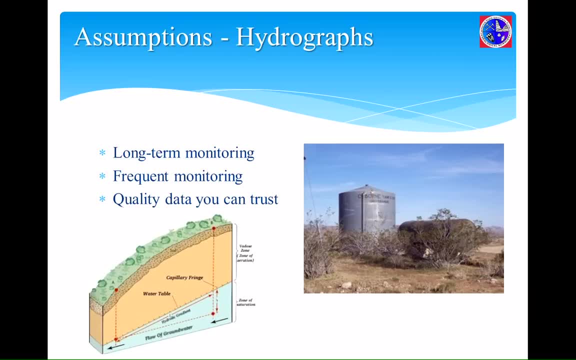 In fact the USGS does a huge website that they measure hydrographs from waters all over the country- Actually all over the world In some cases, And certainly scientists use it. But really we're trying to get lots of data to see what's happening with those water levels. 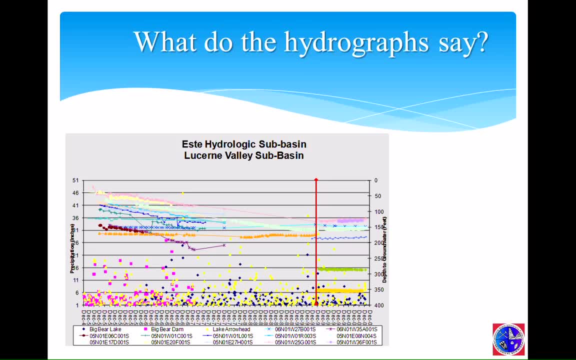 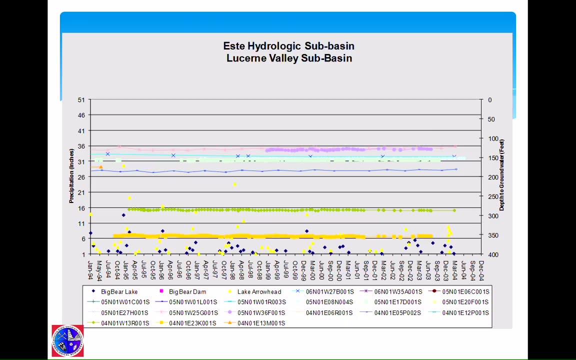 Well, here's that same hydrograph with some other wells in the same basin And they all are showing the same thing: They're all going down. Yeah, there's one anomaly in here where somebody's doing something different, But they're all going down until 1992, I believe it is. 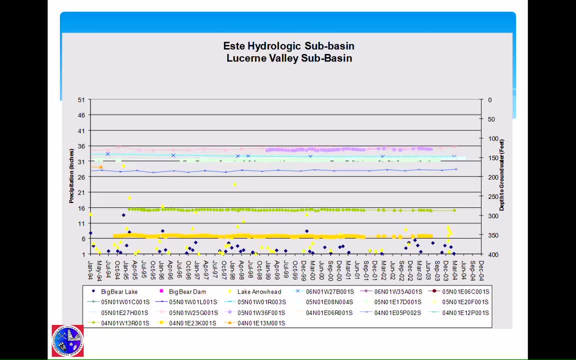 Or 94. And this is that flat area. So, at this point in time, everything was going down until 1994.. Then, all of a sudden, something happened that made it sustainable. Well, what happened was is the farmers out in this area were pumping. 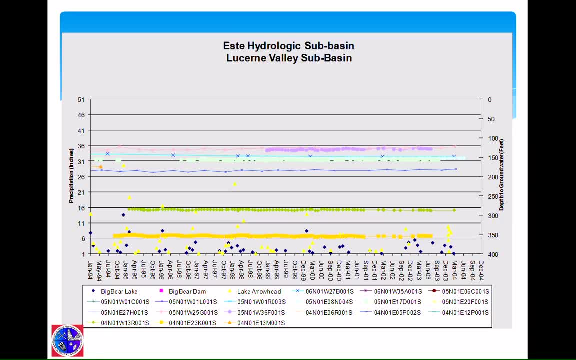 It's Mojave Desert, They're growing alfalfa. Okay, Mojave Desert. What the hell are we doing growing alfalfa out there? They were just pumping out the water. It's easy to get out. It's shallow, Just pump it out. 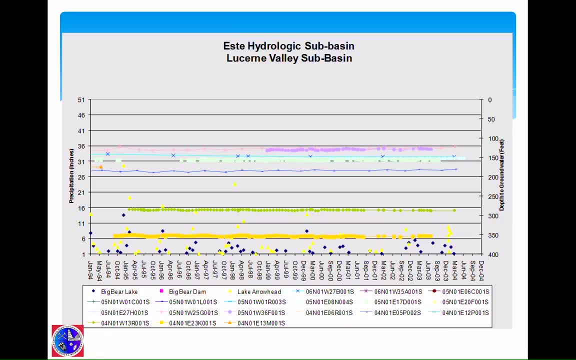 Use it, But they weren't taking care of it, So it was going down. So what happened is they had to come in there And force the farmers, And force the farmers to start utilizing a certain amount of water based upon the water. 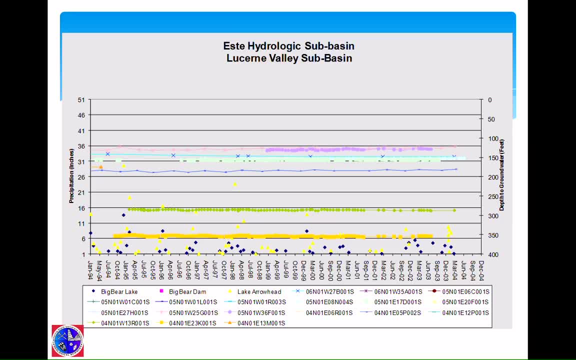 budgets Saying: you just can't keep pumping forever at the rates you are. We're going to ramp you down. We're not going to say you can't water, We're just going to say you can't use unlimited amounts of water. 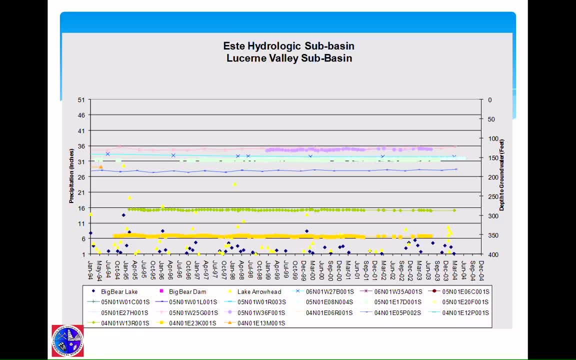 We're going to give you some limits. It's called adjudication in California. Okay, So they went in there and said: this is how much water you get. We're going to divide it amongst the people. whatever they did, And ultimately what happened was is: at that point in time, everyone agreed. 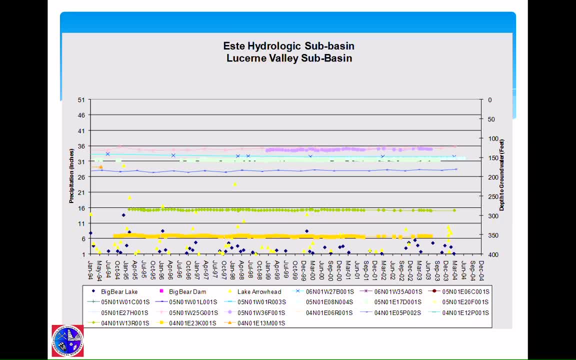 Everyone agreed And everybody was able to live nice and happy with one another, because everything was flat. They used what they were getting. Now, did that eliminate the farmers? No, They just changed farms. Now they grow almonds and olives, Which take a whole hell of a lot less water. 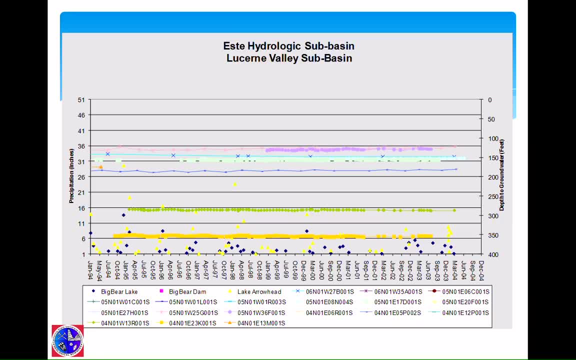 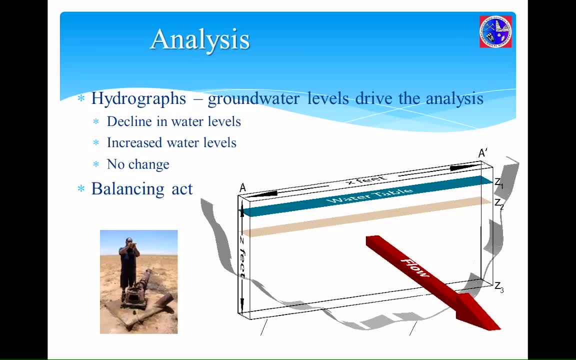 And it turns out, for some of the farmers there- the successful ones- the cash crop was better, So they actually ended up doing a much better job. So, Ultimately, Ultimately, we can use these hydrographs to look at water level declines or increases. 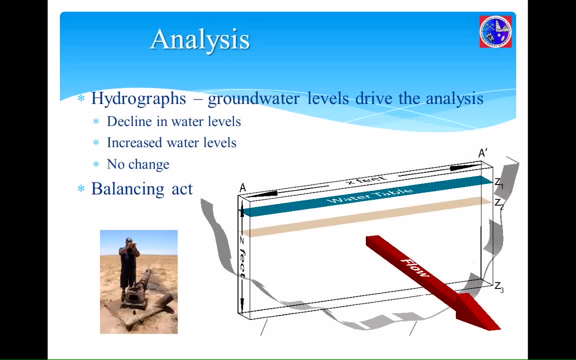 in some cases I've got areas where water levels are going up. Why is that? Because there's less people using it. That can be bad too. In earthquake country, we don't want shallow water tables. Then everything falls down through liquefaction. 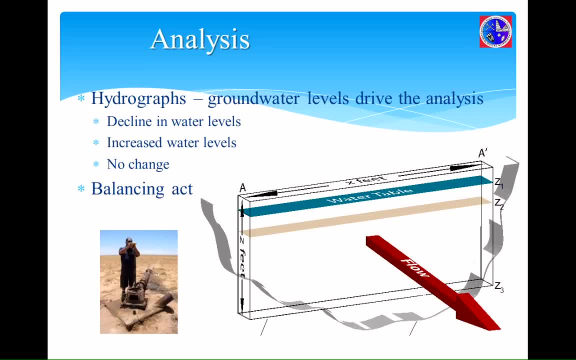 We also don't want you know deep. you know water changes going on in the opposite direction either. So it's a balancing act, But it is one that we can handle. using that simple little equation We can put our water balance. 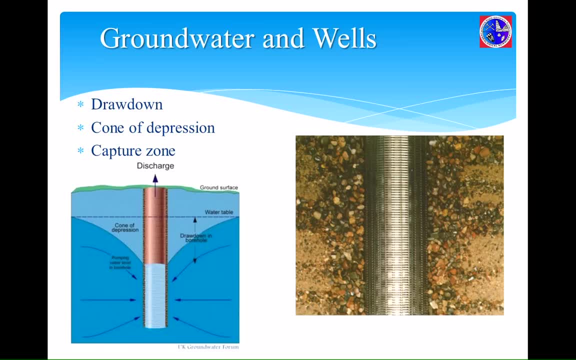 For groundwater standpoint And check So Groundwater and wells. Well, I love this picture And, there again, I'll share this PowerPoint with anybody who wants it. This is a picture I stole from Johnson Screens. Okay, Because I just love it. 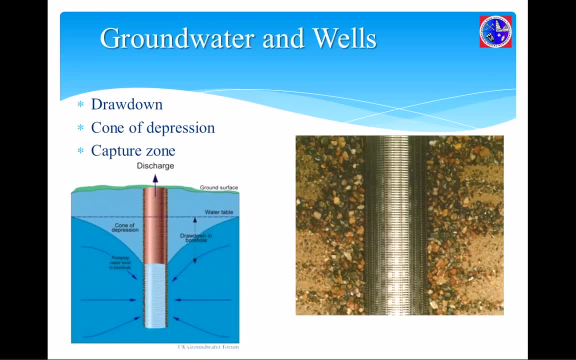 Because it shows what the hell it looks like. downhole, Remember. we can't see it, Okay, But every time we pump we end up with drawdown. What's drawdown? Well, if my water table's up here and I start pumping, I'm going to drop the water there. 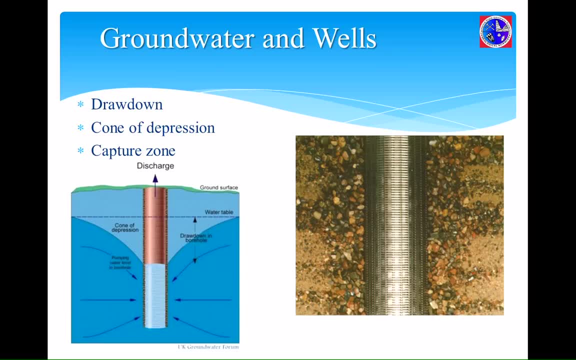 Now the key with an unconfined aquifer is I'm actually dewatering the aquifer, A confined aquifer- when I pump it, I'm depressurizing it, Okay, So I'm taking water out, but the pressure, remember, is way above maybe potentially land. 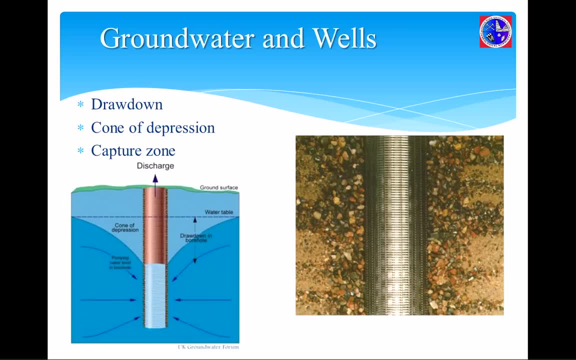 surface. So I'm depressurizing it. I'm not dewatering it Here in an unconfined aquifer. I'm actually taking water out of storage. It's coming out of the geology And this is now part of the veto zone. 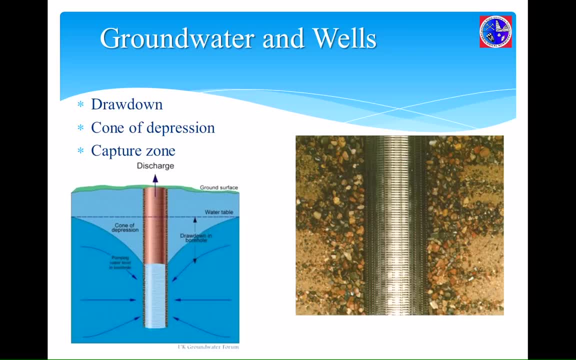 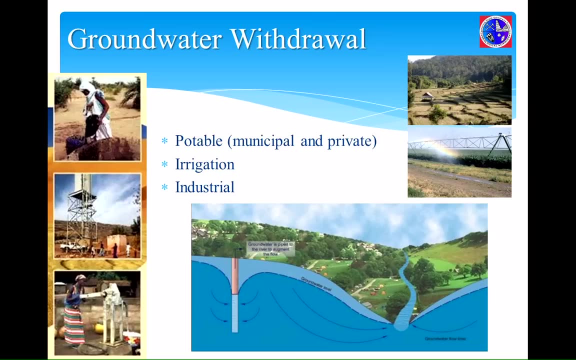 And it could be a permanent basis, or it may be on a temporary basis, And so what happens is we start pumping, Even though our groundwater flow is discharge-free. Okay, We're not charging towards this little creek here, We're basically capturing some of that water which would have gone down here ahead of time. 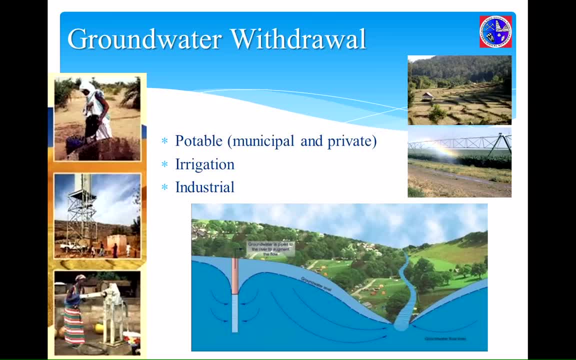 and using it for whatever purposes we want. That is not to say this water doesn't come back in here before here and we have a negative, zero impact, But it can be a negative impact as well. Okay, And this is something that we're going to have to deal with- is putting water wells. 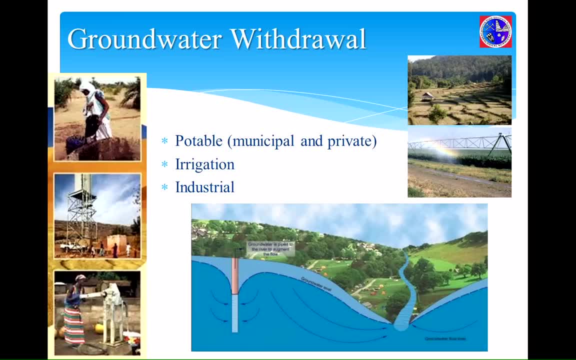 next to streams makes a lot of sense. But if we start drying up those streams, somebody's going to notice, because they can see the surface water. They don't tend to see the groundwater. They don't want to see the water once again. 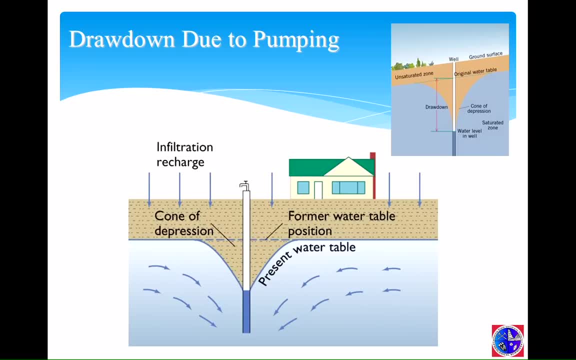 And certainly we use water for all kinds of fun purposes. And here again, if your septic system sits over here, it goes down over back up and you can use it again. What's good about that is what comes out of me can go back in me. 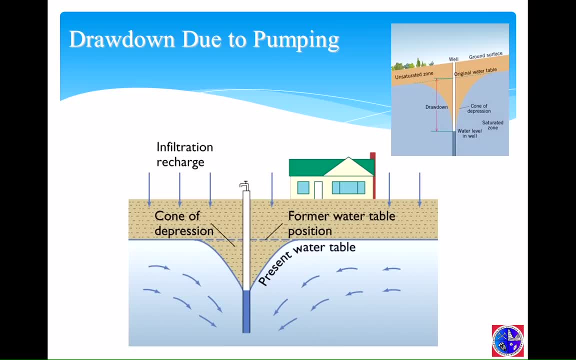 Astronauts have shown that for years. right, It's what comes out of you. I don't want in me. I don't know what drugs you've been doing. Okay, Which is something we're going to have to worry about when I talk about 100 million gallons. 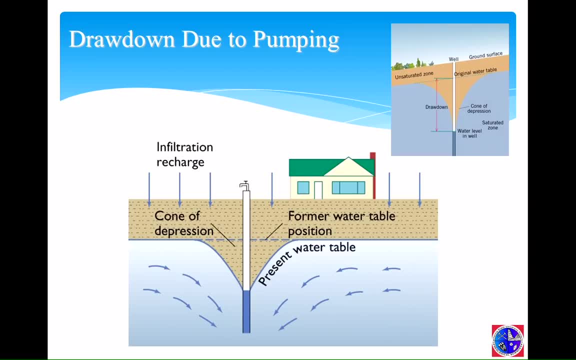 of recycled water every day. One of the things we're worried about is pharmaceuticals. They are small enough to get through the reverse osmosis systems. Now there are such small quantities that you know whether or not it does any damage to us. we don't know. 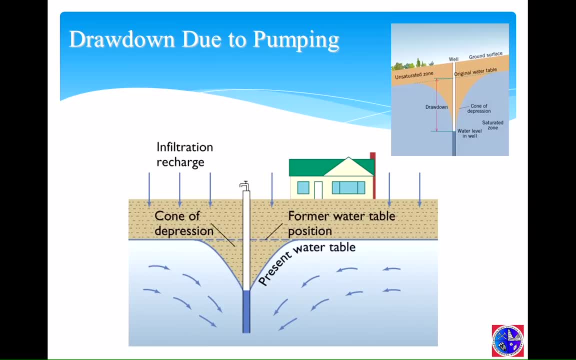 You've got to remember. the EPA sets their standards on all these – on the water quality, but it's based on data from 20 years ago. I mean they're always 20 years behind, So they're risk – they're trying to eliminate the risk with who knows what. 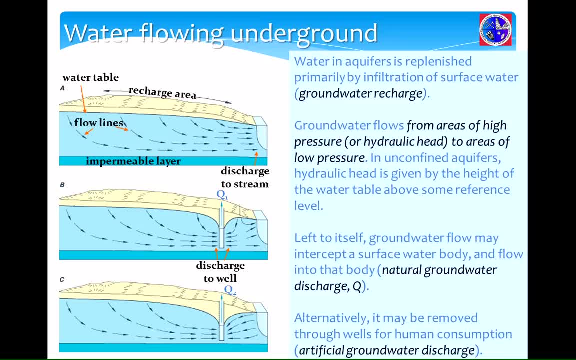 And here's just some pictures real quick. Don't worry about the text, Just kind of showing the flow lines. here is groundwater flow. I have my recharge area up here, a discharge area down here. It could be a stream or a lake. 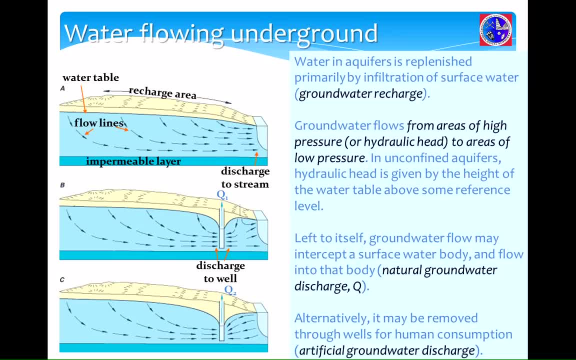 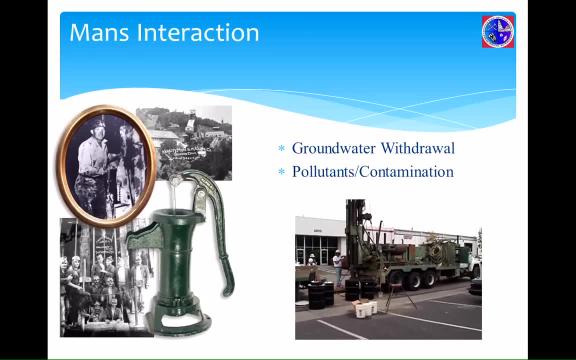 And you can put your well in there and capture some of it, Or you can do it in a sustainable manner and there's ways to do that. Lots of calculations go into it, Man's interaction with it, And the picture I want to show you is this one, right here. 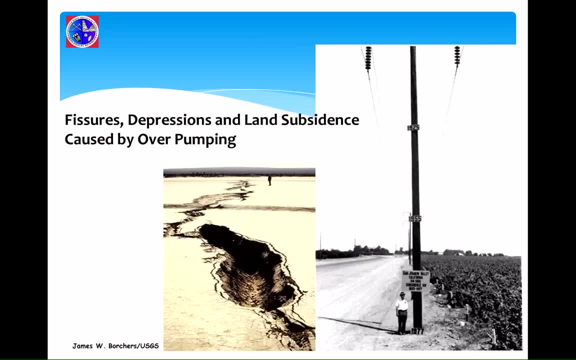 A famous picture: Central Valley of California. What I didn't know until I started teaching was California is responsible for 30 percent of all the food in the United States as a state. Thirty percent of all the food in the United States comes from California. 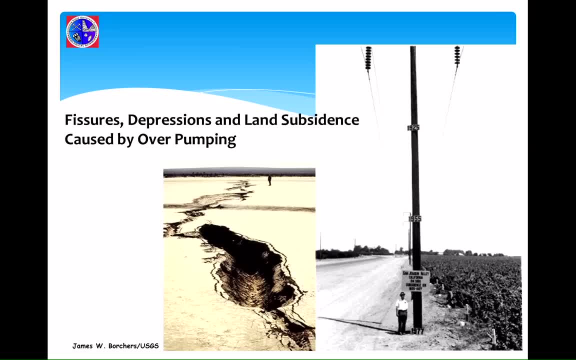 A lot of it comes from the Central Valley 1925, the land used to be up there. Now it's down here. That's not due to erosion, That's due to over pumping the aquifers there and the land subsided. 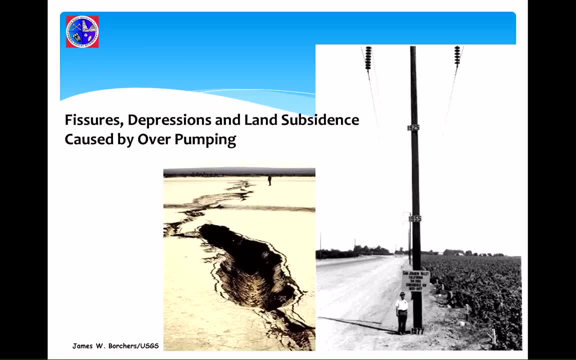 This is an older photograph. The subsidence there has been nearly 100 percent, 100 feet. The land has dropped 100 feet because they took out all the water. There's nothing to hold the sediment up, It just collapses on itself. 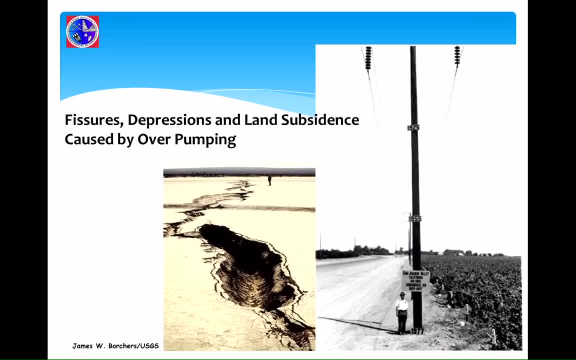 And you can actually, from over pumping and stuff in dry areas, you can get these cracks and fissures going over. But something to keep in mind, And this is not just a California thing: We're seeing this in Texas as well as other states. 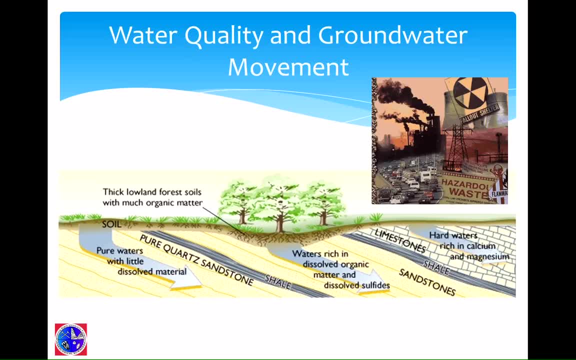 So water quality? Well, when it comes to water quality, keep in mind that groundwater- today you're going to have a lot of water. Water quality today is the cleanest it's ever going to be in the future. It's tough to swallow. 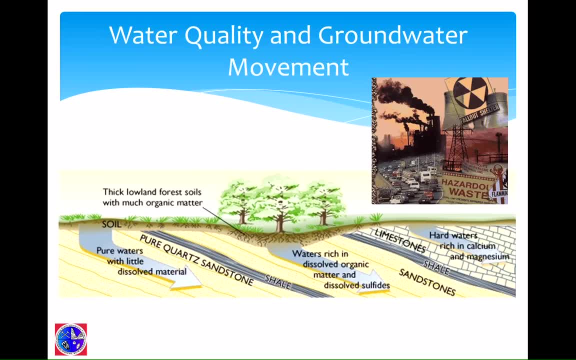 Why is that? Because everybody in this room, everything we do, does something to the water system. Be it you're taking a pill, you urinate the wastewater it's. you fertilized your yard, it's the air pollution that gets in the water that acid rain comes down. 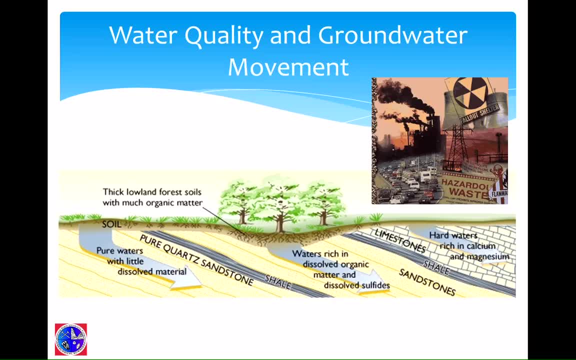 It's always going to get worse. So today is the best it's going to be in the future. That's okay, Because the good news is we have engineers whose sole job is to figure out how to clean this shit up, And their job is to try to provide us with good quality water. 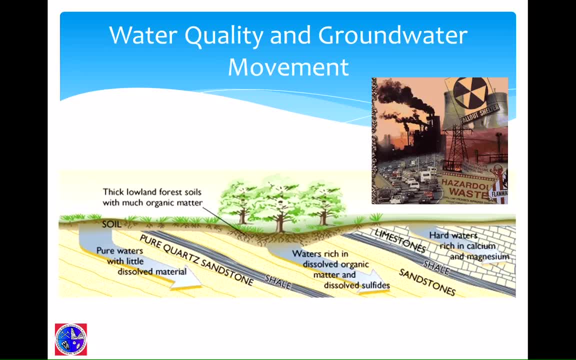 Now, does it mean that we can't get good quality water out of the ground in certain areas? Absolutely, we can. We still do, But over time is that going to stay the same? We have naturally occurring contaminants sitting in the ground. Nitrate and chrome are naturally occurring contaminants. 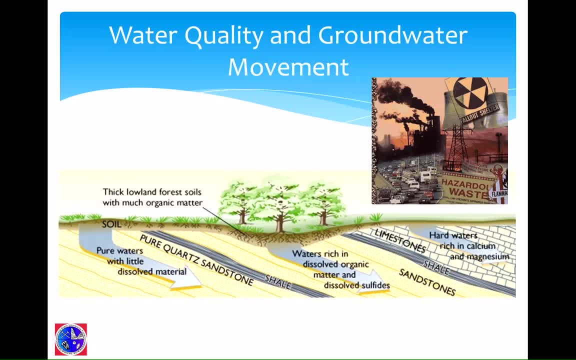 Nitrates are not. Nitrates are man-made. When you find nitrate in your water, that's because somebody put it out there. But yet we have to have the food right, So we have to have the food. So it's a life cycle we're going to have to deal with. 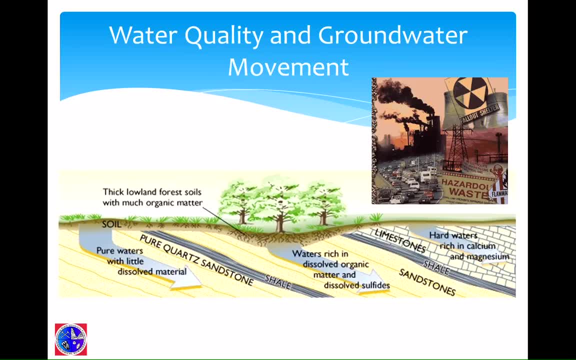 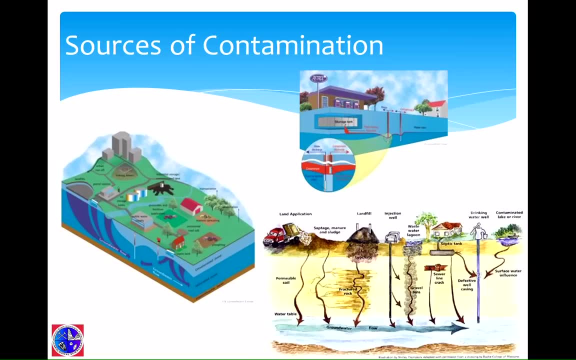 And it can get in the ground all kinds of different ways: Straight down dissolved minerals. obviously limestone can get down there quite quickly. Landfills, Cars, You name it- Everything we do on the surface impacts our groundwater one way or another. 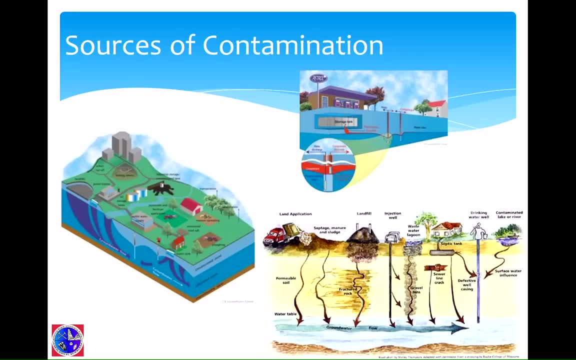 It's only a matter of time, And if you start looking at China and some foreign countries, we're light years away from them from a water quality standpoint. Why? Because we use groundwater an awful lot. We don't rely on surface water. 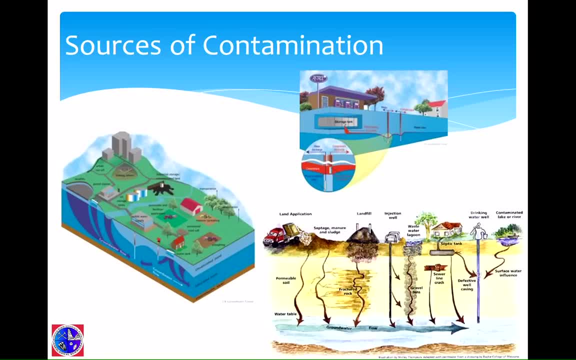 The nice thing about the ground is what It filters shit out. It takes things out, It adds things to it. Why does Orange County and their 100 million gallon recycling? why does Orange County and their 100 million gallon recycling? why does Orange County and their 100 million gallon recycling? 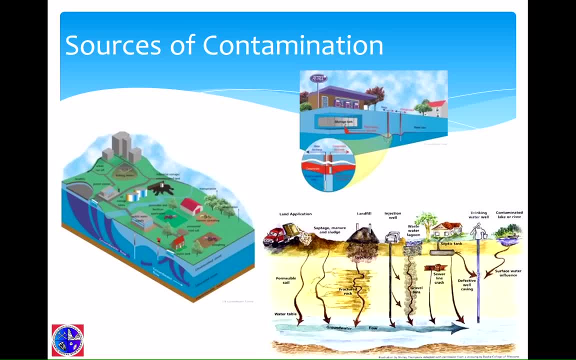 gallon recycled system, put it back in the ground. Anybody know Why don't they just give it to us? Because when it comes out of their treatment plant, it's pure H2O. It has nothing in it. Pure H2O- if that's the only source of water you drink- will kill you. 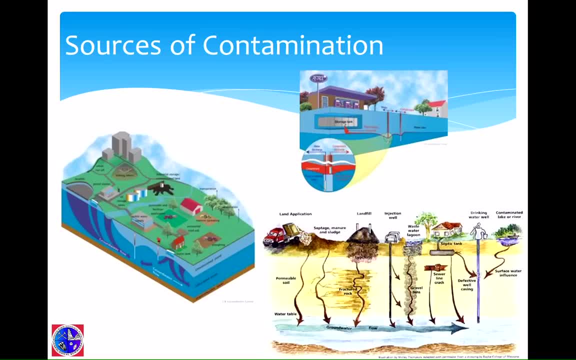 It demineralizes you. We need the minerals, We need the geology in order to put the minerals back in the water. so when we drink it, it has flavor. Distilled water has no flavor because there's no minerals in it. It has no contaminants either, but that's okay. That just adds flavor. 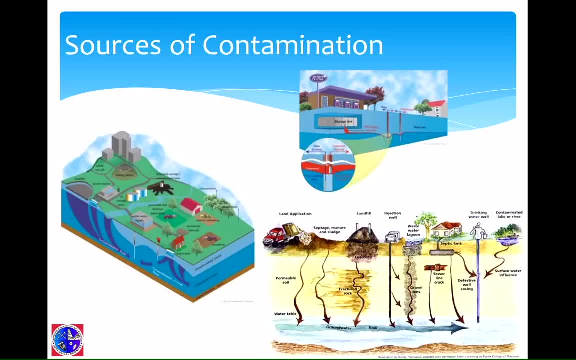 So we need that geology, We need that groundwater or that water to go into the ground, dissolve some of those minerals, pick them up because we need those. This is a human being. Remember: the only thing we are is a little pile of white stuff after you get zapped. Remember the. 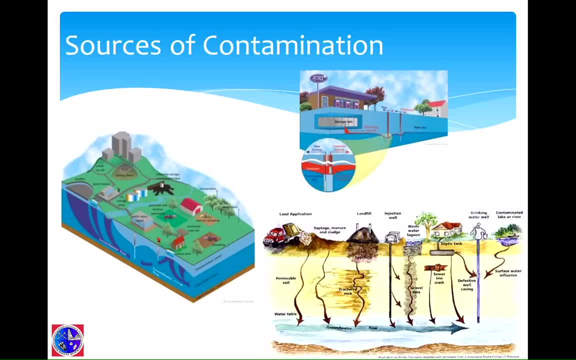 old Star Trek, When they zapped the guy and the only thing left is a little pile of white stuff. All we are is jellyfish with salt. Well, that's what we need. So we need that water to go back in the ground. So groundwater is always. 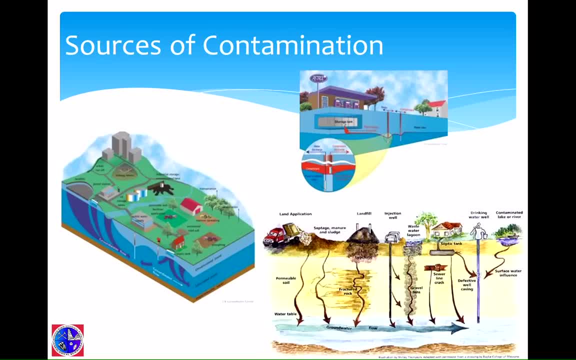 going to be a great source of drinking water. Why does surface water suck so badly for drinking water? Anybody know Well, I mean, it's always going to be slightly acidic, but that's not really the problem. What is it? It has low mineral count and it fluctuates. It's at the surface. 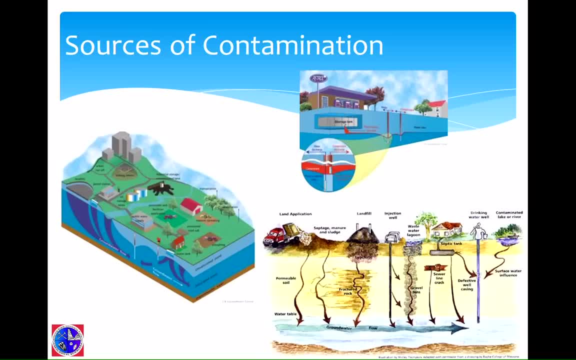 So flow-wise it fluctuates a lot more than groundwater. Groundwater is pretty steady. The other thing is it doesn't take a whole lot to contaminate surface water. It actually takes quite a bit to contaminate groundwater, So groundwater is always going to be a safer source of water. 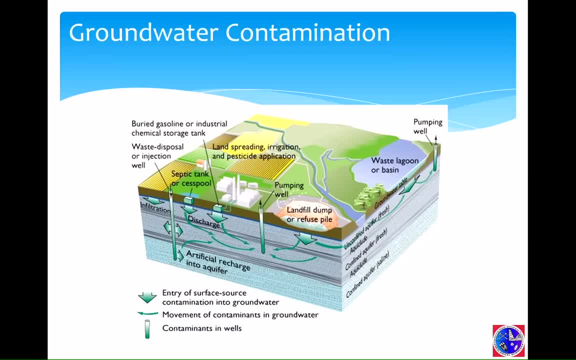 ultimately, Certainly, we're going to have land farming and all that good stuff. Landfills are always easy to point out, Factories are always bad things, but we all like our iPhones and everything else You know. I point out there's a seven-mile plume of TCE under City of Phoenix. Why? Because somehow, 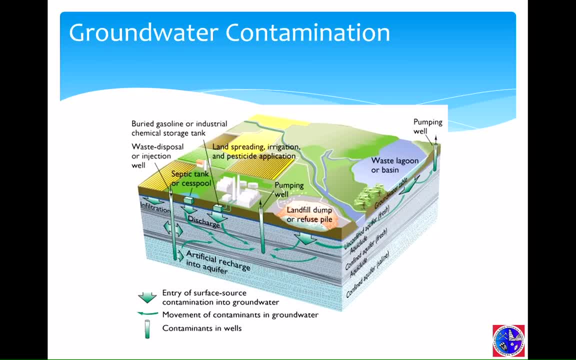 City of Phoenix wants to make a lot of transistors, But every transistor requires 170 to 180 gallons of pure water. It's in Phoenix, Arizona. Why wouldn't we put this in the tropics, somewhere where they actually have lots of water? You know, 180 gallons per transistor. Now how many. 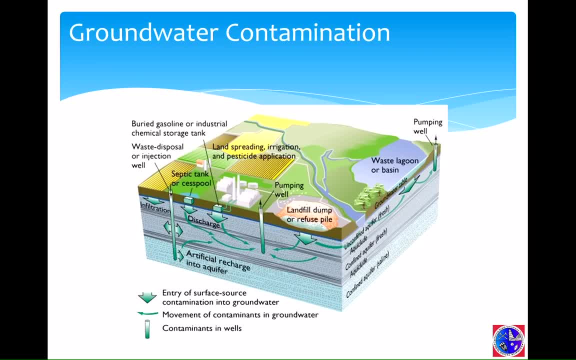 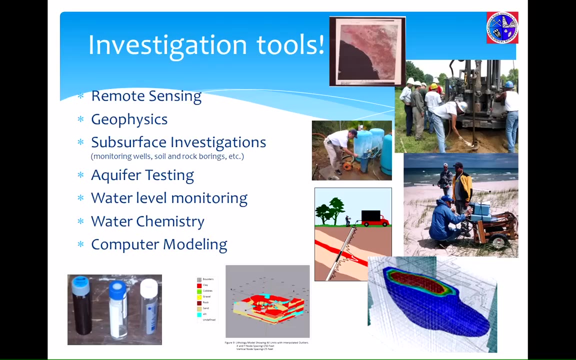 transistors in your cell phone. Yeah, every cell phone. I mean you add it up, I mean we're talking thousands of gallons of water just to make one phone, And it's in Phoenix, Arizona. You know who knows. 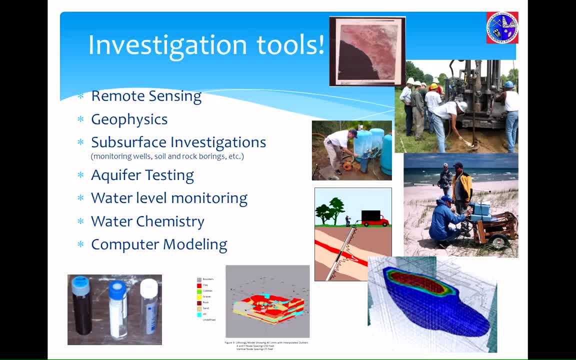 Some tools we use to investigate things. We're starting to use remote sensing a lot more. I can't wait to get my own drone. You know it's like drop bombs and ex-girlfriends or ex-wives, whatever it is, But nonetheless I want a drone. That's just cool And we're 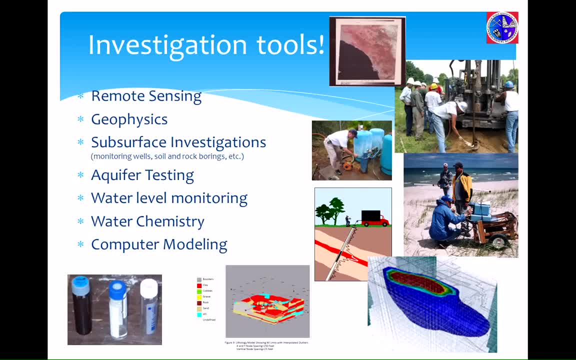 going to get our Amazon's going to deliver all our packages by drones. now You order it in 30 minutes, The little drone flies to your front doorstep, drops your book and off it goes, Right. So it's going to be cool. 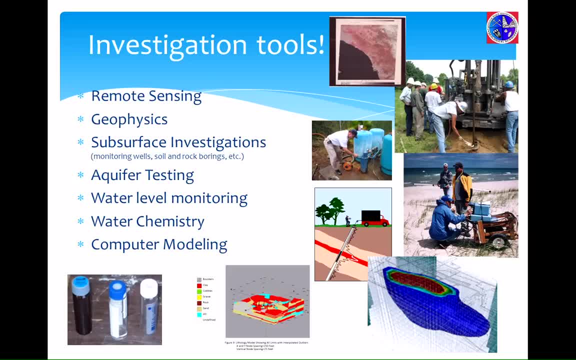 It's going to be some fun things, But we use geophysics. Here's some geophysics out on the beach in Lake Michigan. We're looking for some clay units for discharging to Lake Michigan. A lot of computer modeling is taking place now which is allowing us to do some things There. again, the problem with it. 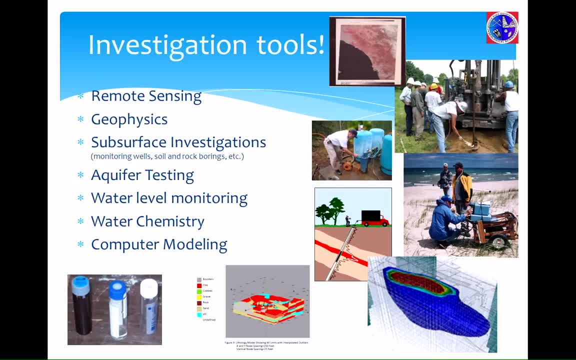 is it's only crappy data, You can make a pretty picture, but if it's crappy data it doesn't mean any much. But there's going to be a lot of advancements here over the next, you know, decade. It's going to be kind of. 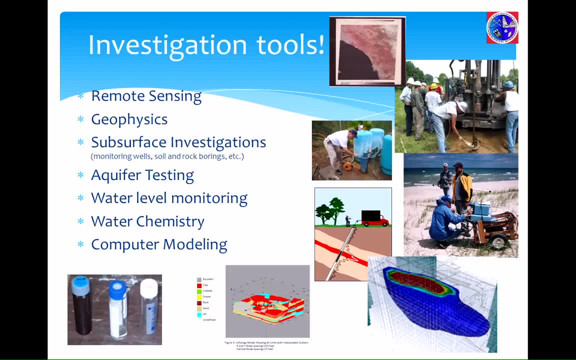 fun And I, like I said I the drone thing is something I'm excited about. In fact, I have my own blimp, by the way, And I've had one for twenty years. That's how I've been taking. 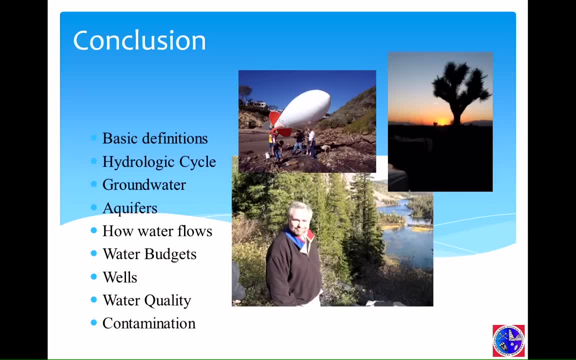 my aerial photographs. So actually I own my own blimp. How many people do you know that? How many people in here own a blimp, See Special Um. so anyway, hopefully you learned something about. you know basic definitions and some water quality and some. 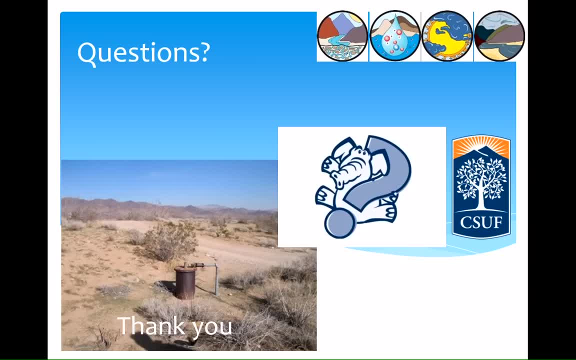 other things. We went through some things somewhat fast, but nonetheless, I want to thank everybody and thank Cal State, Fullerton and NJWA for allowing me to be here, and I appreciate everyone's time and thoughts. Any questions besides the code? Yeah, Any questions? Yeah, go ahead. Yeah, the Oklahoma is being depleted at a rate that is also causing it to collapse Absolutely, And that will never be resolved. We can take steps to start replenishing parts of it, but overall we're probably not going to gain it back unless climate changes again and which gets rainy, which? could happen. I mean, it was an old sea to begin with so you know, maybe it comes back to be in that, Maybe you can get some ocean side property there. But certainly there's things we can artificially do to recharge Some of the things people are doing a lot more. What Orange County does was a gamble. We 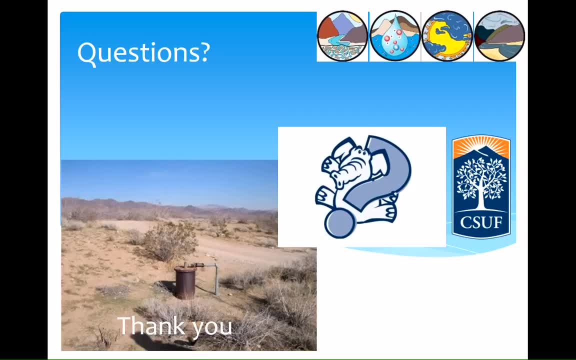 spent four to five billion dollars to set up this system- And I think that's a good example of that- And had to go through all the EPA and everything else and it was just amazing. But now they've gotten to the point where they've proven. 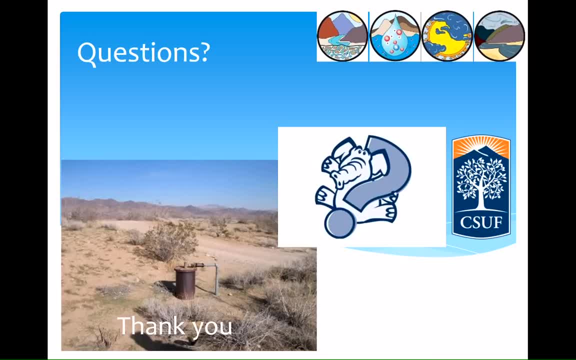 beyond any reasonable doubt, and other countries are modeling this too: Singapore, their whole system is designed after Orange County, Saudi Arabia, everyone else. And that is it's taking the water that we use, for whatever purpose- I mean, I talk about wastewater and toilet water. It's 48 hours from the time you flush your 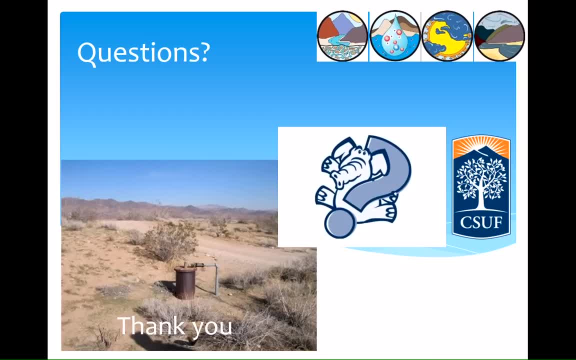 toilet to that water drop, being back in the ground 48 hours. So that's going to take a lot of time And it's going to take a lot of energy And it's going to take a lot of energy to get it back to where it was before. And if we do that, ultimately during the wet years, in order to become sustainable. the wet years will fill things up if you can become sustainable in the short cycle. From farming standpoint, we have a lot of return flow. Now we're getting better about it, because that's one thing: When we farm, we're always over water. 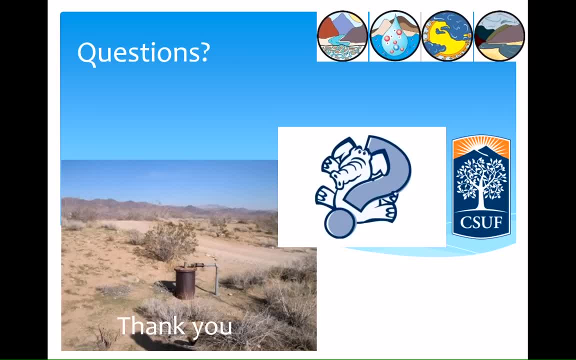 Because more water is going to make it greener. Well, this isn't always the case. So the farmers have done a better job now of managing the soil moisture, So they are managing that a little bit, And that should help bring some stuff back. 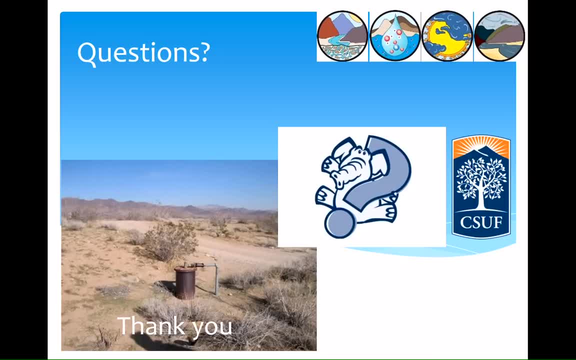 But ultimately it would be more of this urban water cycle than wait for the wet years to bring back things to a bigger, fuller situation. So, yeah, Other questions, None. Anybody asleep yet? Yeah, I don't understand. Do we take nitrogen and actually make water? Yeah, Every time you sweat, Like me right now. I've got lots of H2O in these modern pits. Is that not an answer? Well, the problem is it's economically. It comes down to economics Like desalination. We live in California. We've got the world's largest ocean sitting right there. The Pacific Ocean. Why won't we just take the water from there, get rid of the salt and use that for drinking water? And we are. The problem is from a cost standpoint it's about well. in 2000 it was about $2,000 an acre foot to treat desalinated water. We could buy water from anywhere else in the country for about $1,000 or less. We stole from the Colorado, We steal from San Francisco. We could buy Lake Michigan for cheaper than that. Now, Michigan passed a law that we can't- California- specifically California- can't steal the water, by the way, Why they had to pass a law for that, who knows. But they did. But now the desalination is about $1,000.. What Orange County is doing is about $900 an acre foot for its whole system. So we're still cheaper than that. Sooner or later desalination price-wise will get down where it makes sense. 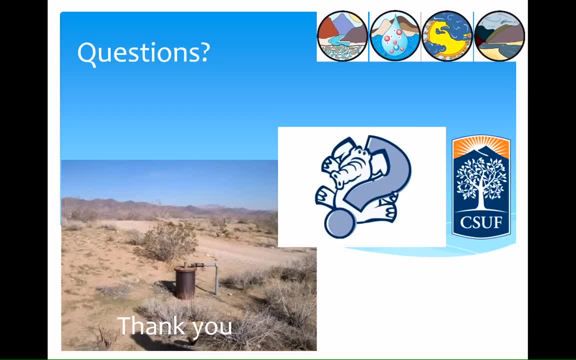 But, from an energy standpoint, is where it really costs. And so, just like making H2O, Yeah, we can make it, We can have hydrogen cars. Why don't we? You know, because of cost And it's just over time. 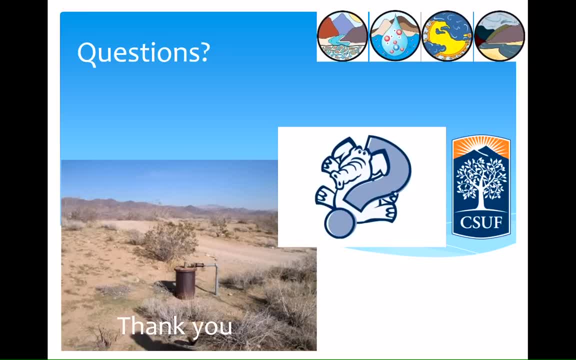 Worse as we can move forward. That means there's going to have to be a cost to water. Water is free. You only pay for delivery. Now you pay for some treatment of the water, But you're actually not buying the water. You're buying the delivery of the water. 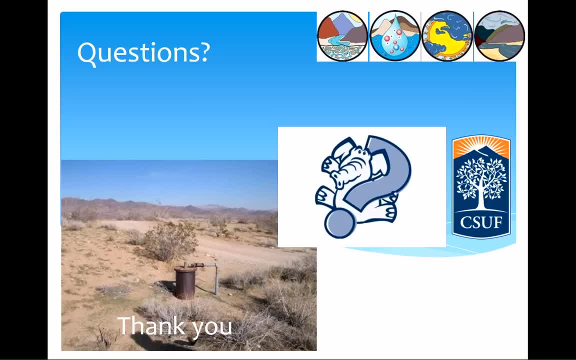 And, of course, my wife's, one of those people. We live in the city And she complains about the taste of it all the time. Ah, I taste the chlorine. Why do we put chlorine in water? Well, it keeps all the bacteria from killing you. It kills all the bacteria, Not in their pipes, Not the city's pipes. Their pipes are fine. It's your house. Where's the worst spot for bacteria? for water, At your faucet. What's the worst kind of water you can ever get? 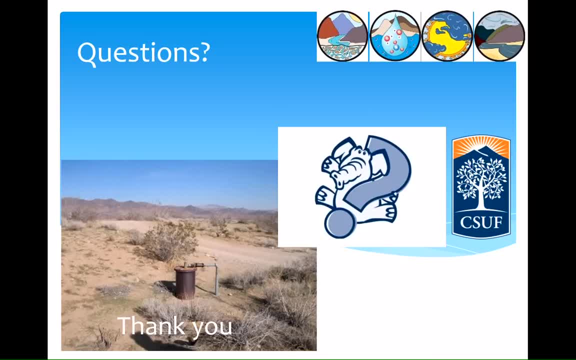 Take a five gallon jug down to your local grocery store And that big thing out in front. It's attached to a garden hose, by the way, There's tons of bacteria there And yet people are still sitting there buying their five gallon bottle of water. Because it has to be good. It came from the grocery store. We pay as much for water as beer. At least beer is distilled And I get happy over it. I need t-shirts. Drink beer, Not water. So back to Orange County, Yep. And the reformation process. How come more cities aren't doing that? Is that the cost effectiveness that you mentioned Well, and it also depends on where you're at. In Orange County we have four million people and we're a desert. We only get 16 inches of rain a year, So it made sense for us to be more of that system. If you're in Minnesota, up until this point in time they had 10,000 lakes. There's plenty of water, So they don't need to do it. 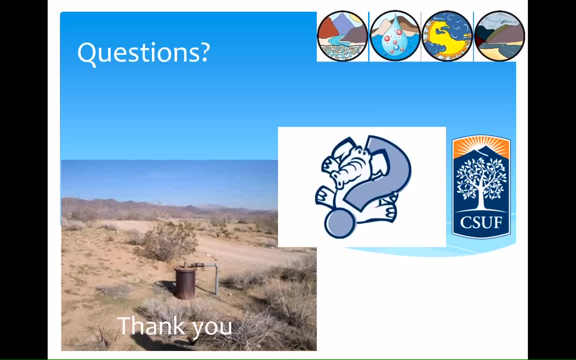 I mean Atlanta Georgia. I mean the river that they ran the Olympics- the kayaking I guess in is dry. There's no water in that river anymore. They could not run the Olympics today in Atlanta Georgia. And it's because they dropped all the water. They stole all the water from the river and had fights with other states and other things. There's a lot more to it, But again they're looking at recycling stuff. It's why Coca-Cola is doing a big push on trying to do water recycling. 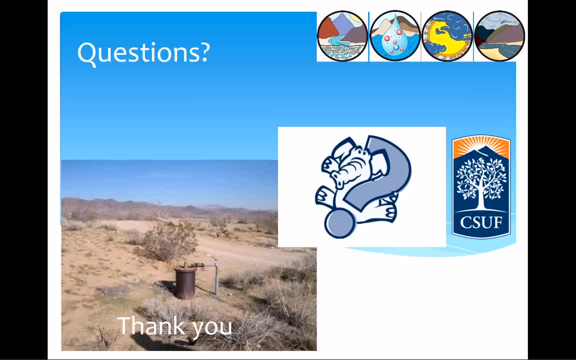 You know, recycle the plastic bottles. I mean the same thing holds true for water as for trash and everything else. I mean. I hate to use the word sustainable, because 99% of the public doesn't even know what the hell it means. 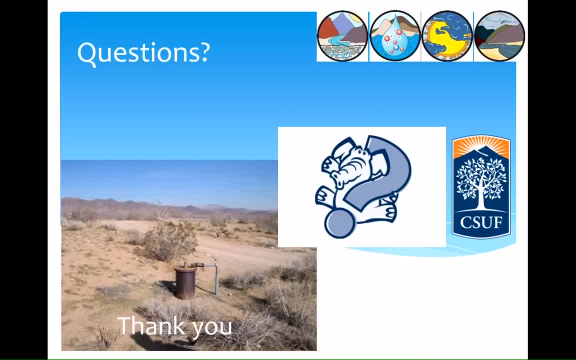 It's a cool word, It's sexy. I can write sustainability on any grant and get it. It doesn't mean it has anything to do with sustainable. But when we use 100 gallons of water and we don't have to buy it from anyone else, we are now sustainable. There's a cost to that, but we are not having to borrow water from anyone else. Other questions: Someone else had one.